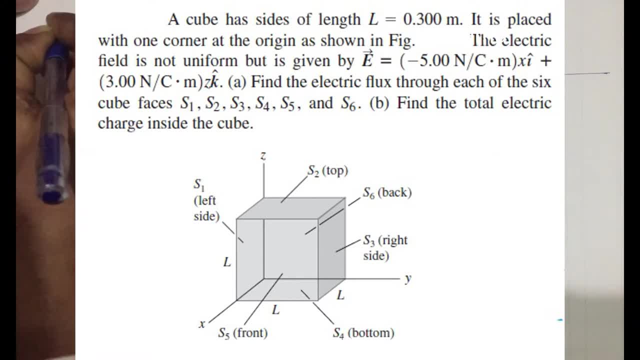 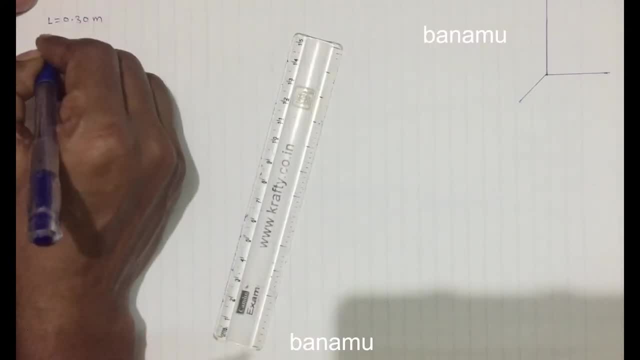 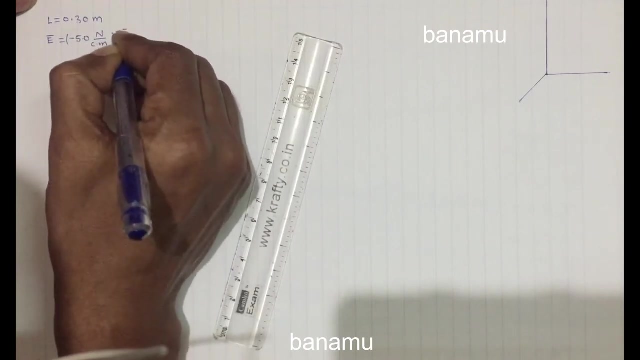 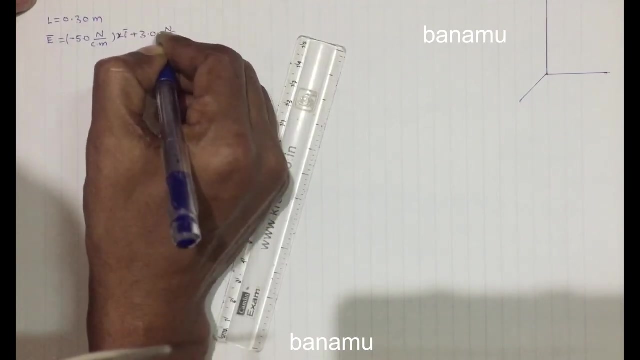 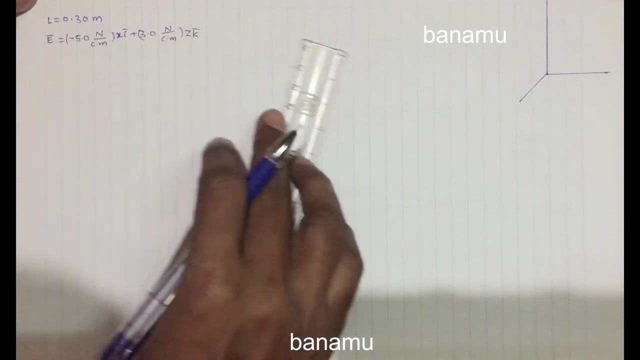 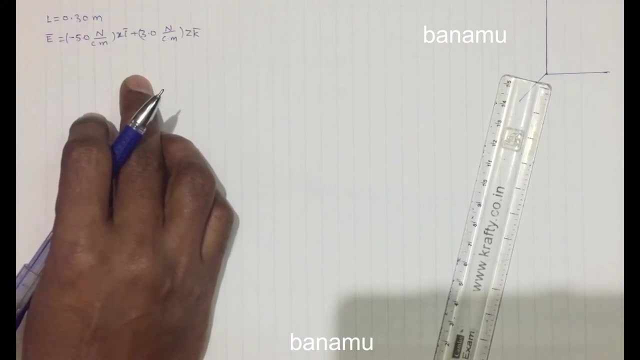 length L is equal to 0.3 meter. The electric field E bar is equal to minus 5 Newton per Coulomb meter into X i bar, plus 3 Newton per Coulomb meter into Z k bar. This is the non-uniform electric field. We can calculate the electric flux at the each. 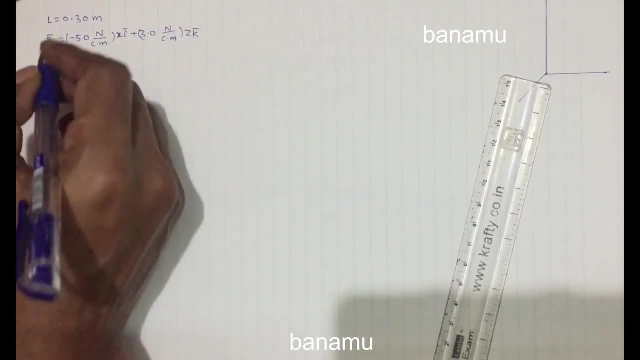 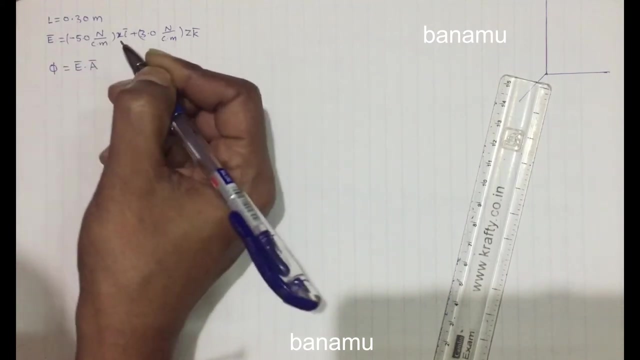 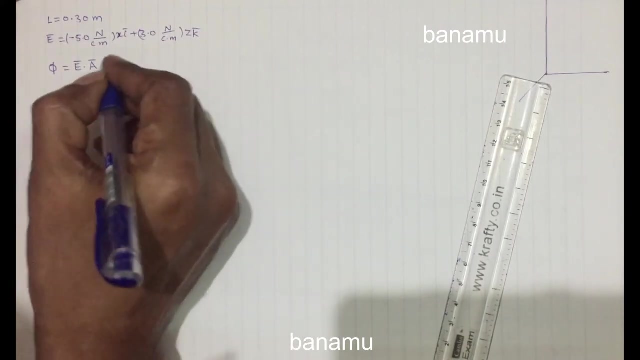 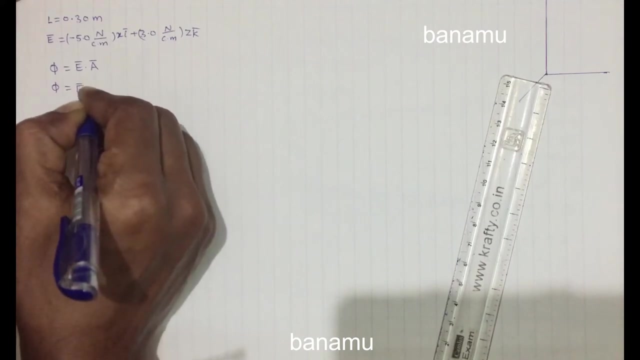 surface. So the electric flux phi is equal to E bar dot, A bar, where E is the electric field and A is the area of the surface. So the electric flux phi is equal to E A, n cap, where n cap is the unit normal vector. So where n cap. 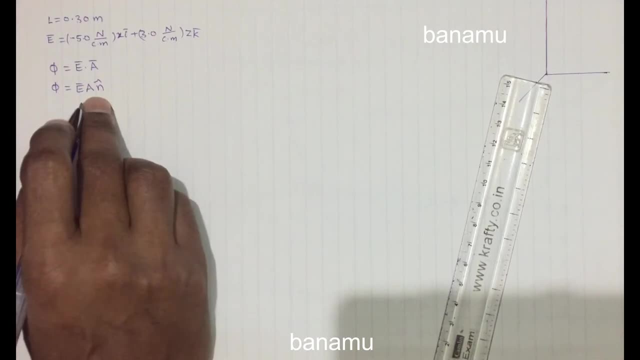 Is the unit normal vector. So The surface area of the unit normal vector is illimitated by the direction x or any of the previous cases, the. the area of the unit normal vector is illimitated after a dimension. i Now try to find the electric reflectance. 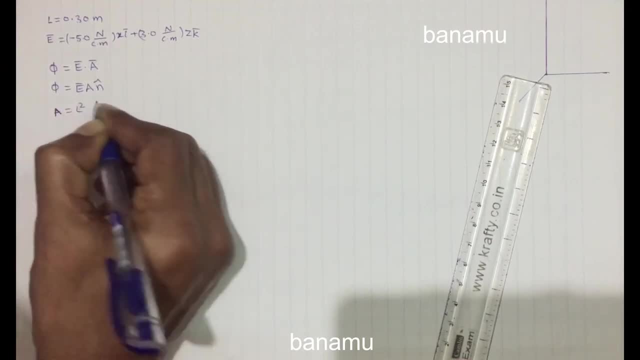 by looking at the Desk Principal from z laughter. Let us draw a Were Lythus there and see that as this classical. You know the three D FC, articulate terms, parameters are present in the work. there is a minute and time constant and L square A is equal to where L is the 0.3 meter, So 0.3 meter whole square, The area. 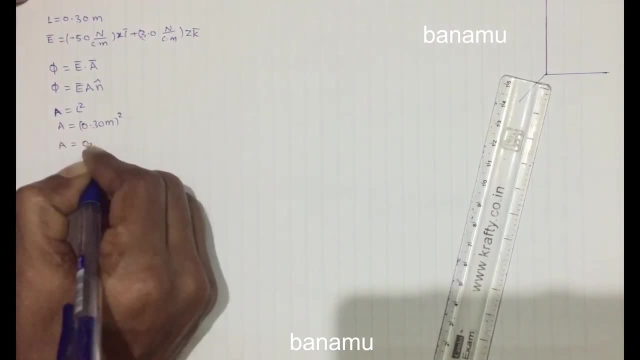 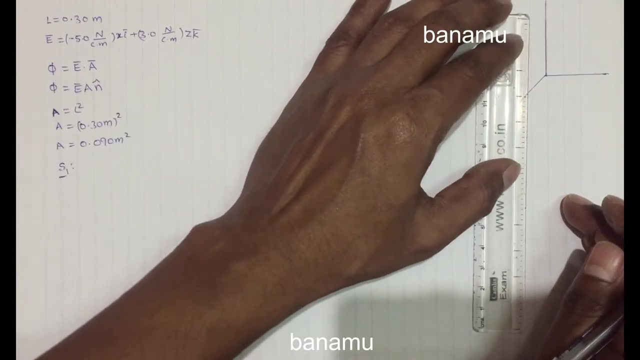 of the face A is equal to 0.09 meter square, So this is the area of the surface. First of all, we can calculate the electric flux at the surface 1.. This is the surface 1 or left side of the cube. Let us draw the surface 1.. Let us draw the surface 1.. This is the 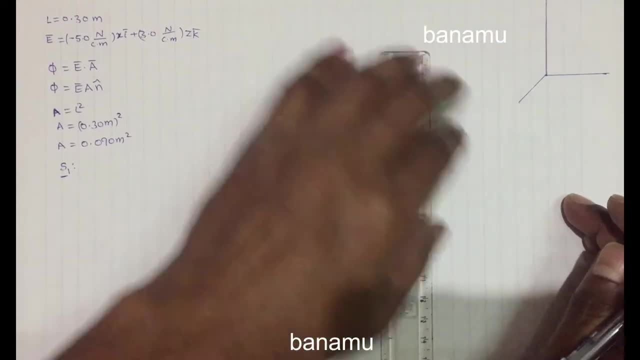 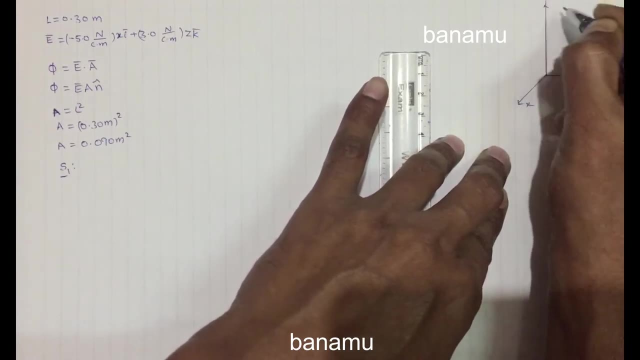 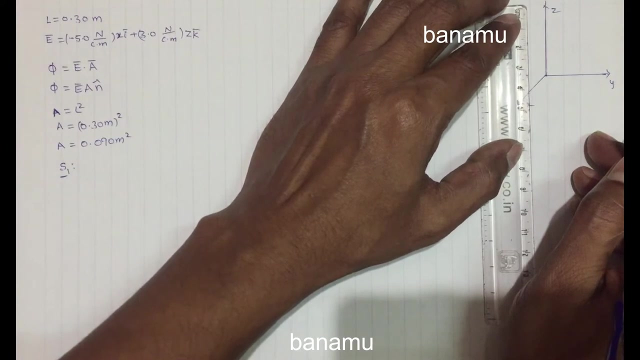 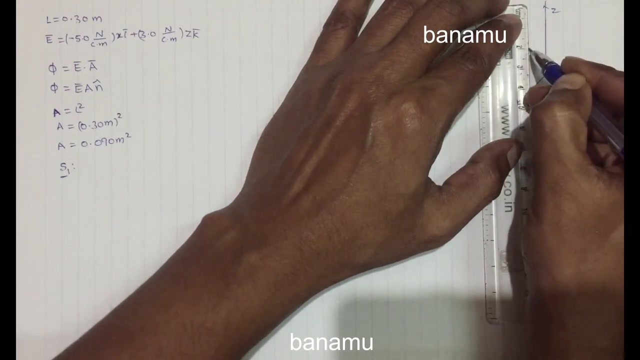 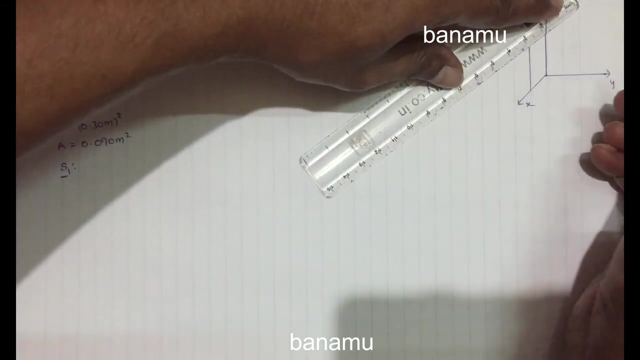 left side of the cube. So let us take this is the x axis, And this is the y axis And this is the z axis. So let us draw the left side of the cube, surface 1.. So this is the left side of the cube, This is the surface 1.. This is 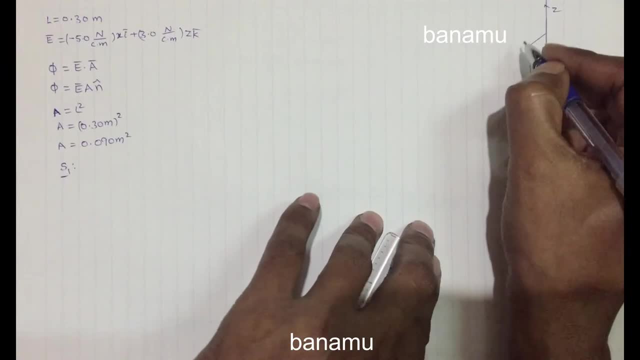 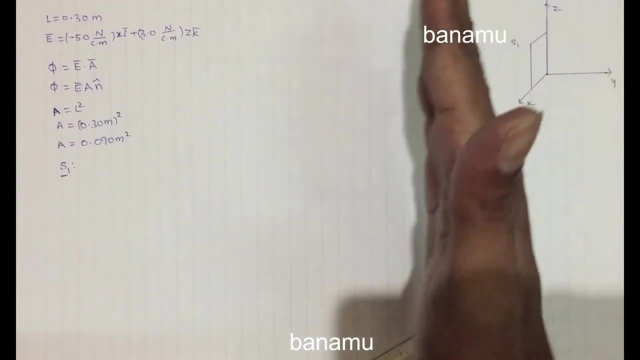 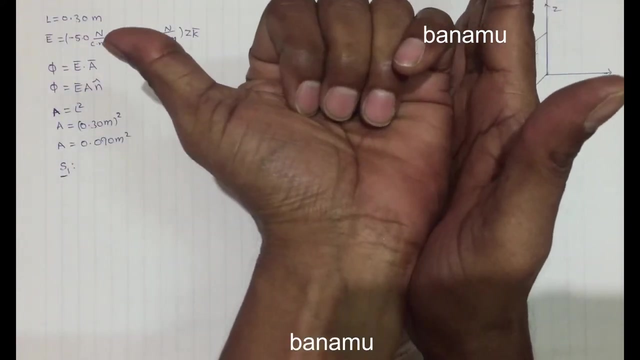 the surface 1.. This is the surface 1, or left side of the cube. Do not forget to notice the x axis. Then learn this: tested the x axis and this is z axis. Do not forget to notice the 0 axis. 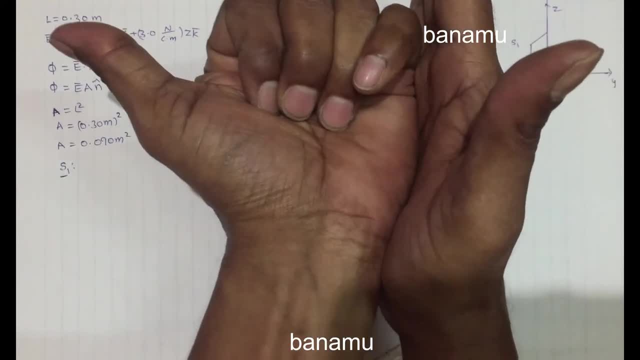 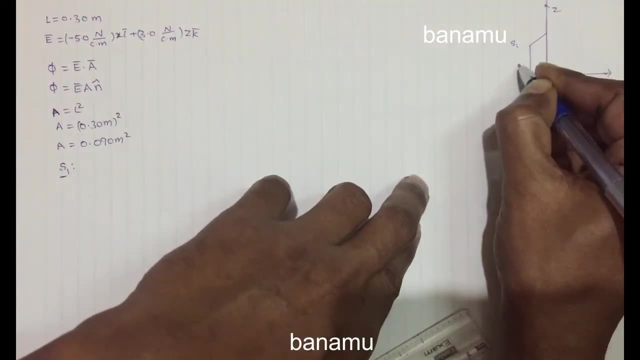 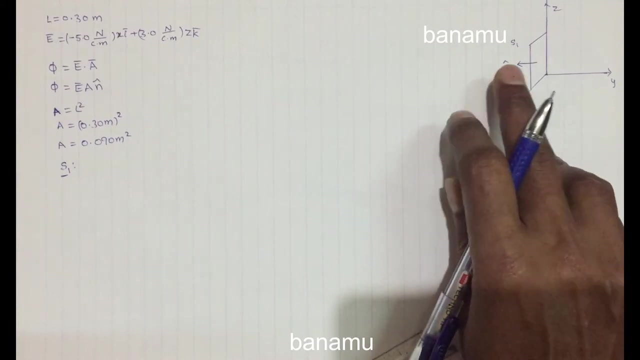 So this is the surface 1.. So let us take this surface. This is the surface, The unit surface S1. So the direction of the area, unit normal vector along the negative y direction. This is the n cap S1, n cap S1.. So the n cap S1 along the negative y axis, So n cap S1. 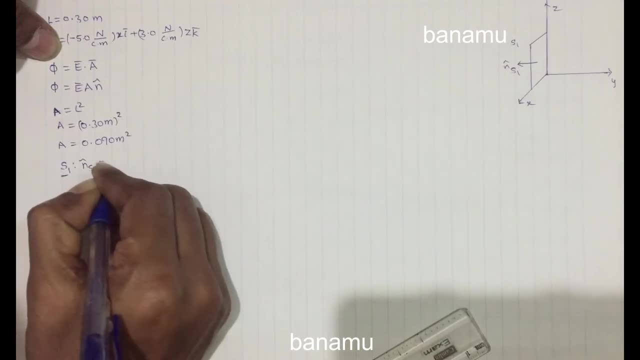 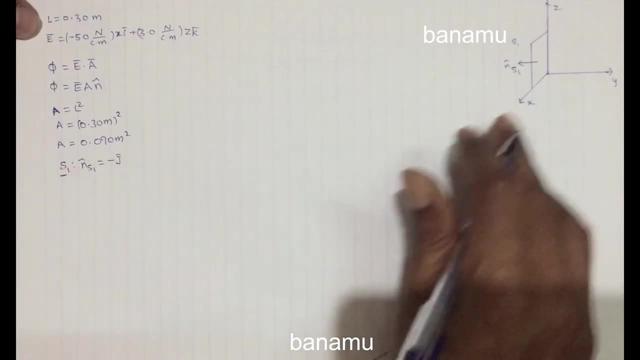 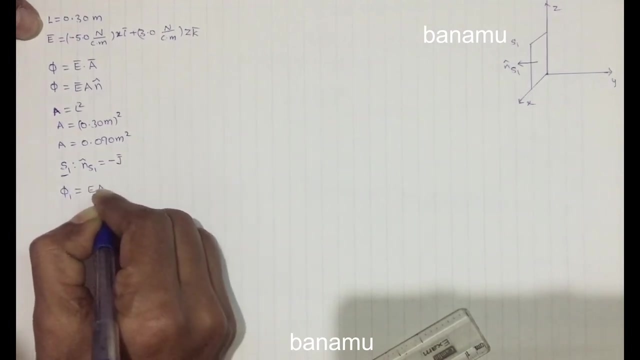 is equal to n cap. S1 is equal to minus j bar. So the electric flux at the surface S1 is the phi 1.. Phi 1 is equal to E a n cap S1.. So phi 1 is equal to the electric field is. 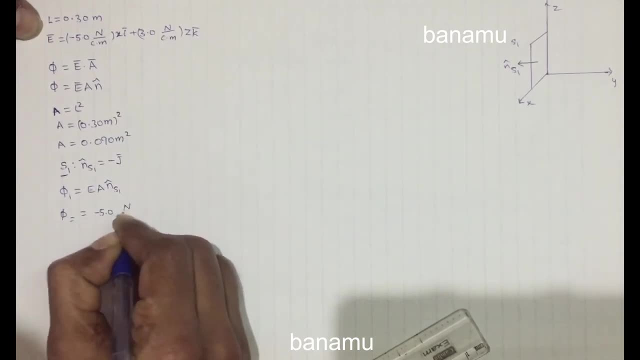 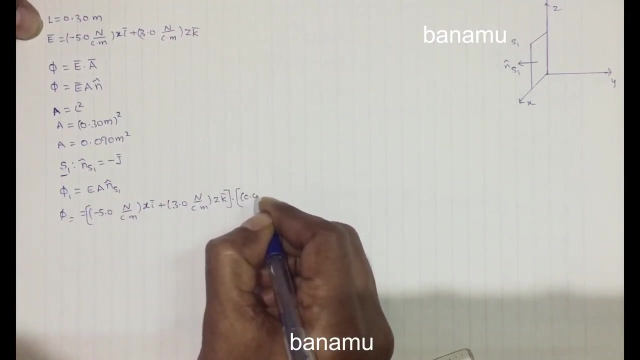 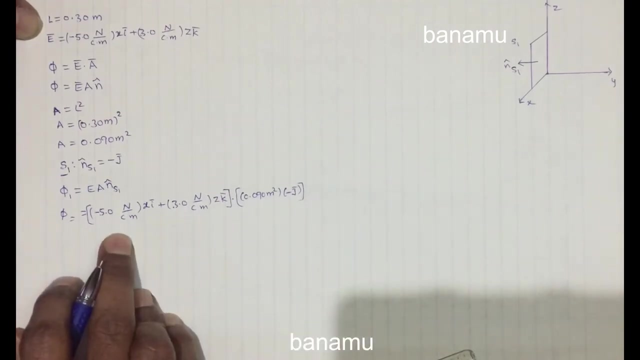 the minus 5 Newton per coulomb meter. This is the electric field dot. The area is the 0.09 meter square into along the n cap is the minus j bar. So the dot product of the two vectors is: phi 1 is equal to i bar. dot j bar is equal. 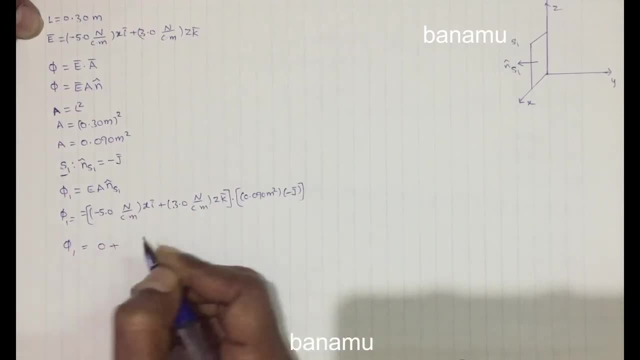 to 0 plus. and the second one is k bar dot j bar is equal to 0. So the electric flux at the surface S1 is the phi 1.. Phi 1 is equal to 0.. This is the electric flux. And consider the surface S2 or top of the cube, Consider the. 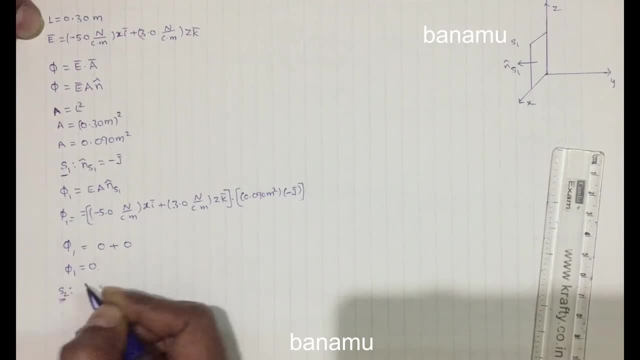 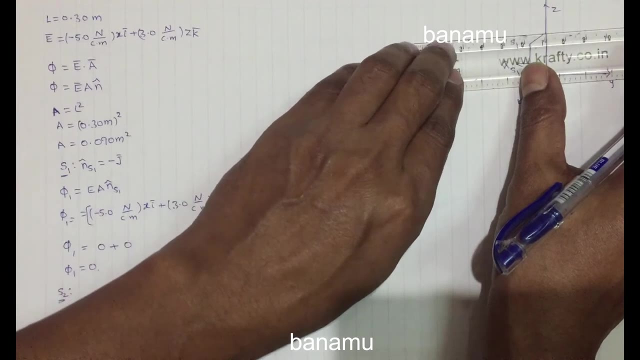 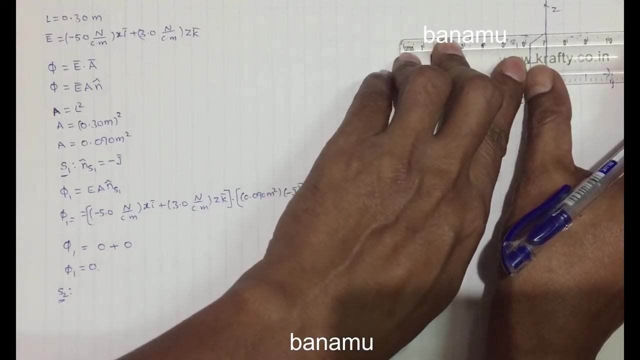 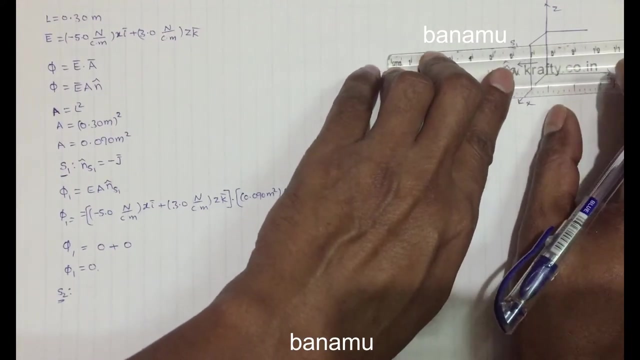 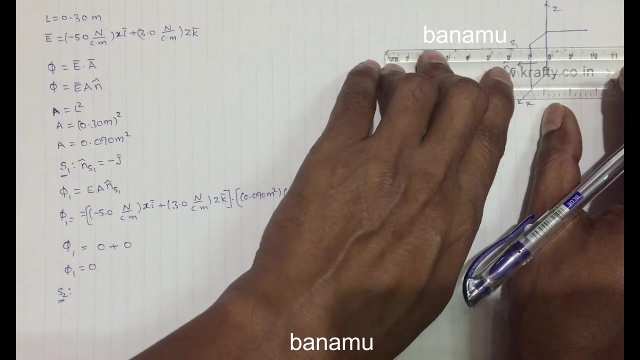 surface S2.. Consider the surface S2.. Draw the surface S2.. Let us draw the surface S2.. The surface S2 is the top of the cube. This is the surface S2.. This is the surface. S2 is the top of the cube. 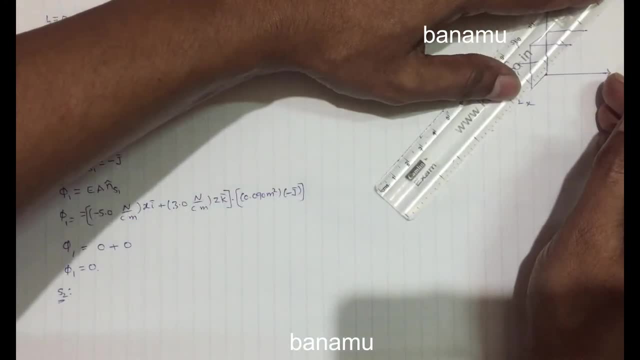 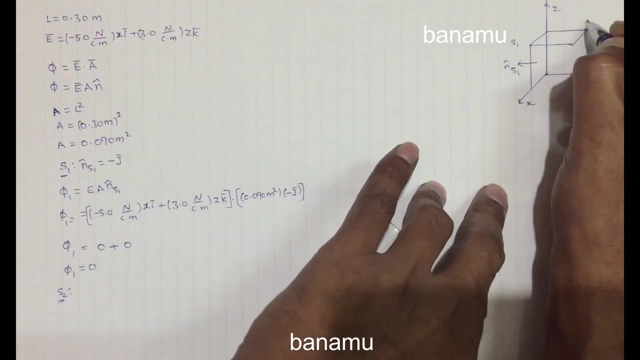 So the surface S2, we can draw the unit normal vector with the surface S2.. This is the surface S2.. The surface S2 is the top of the cube. This is the surface S2.. This is the surface S2.. 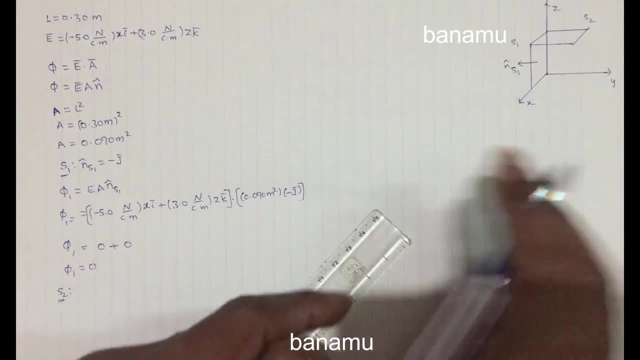 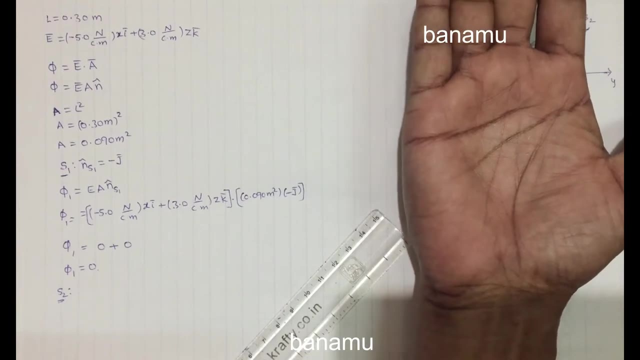 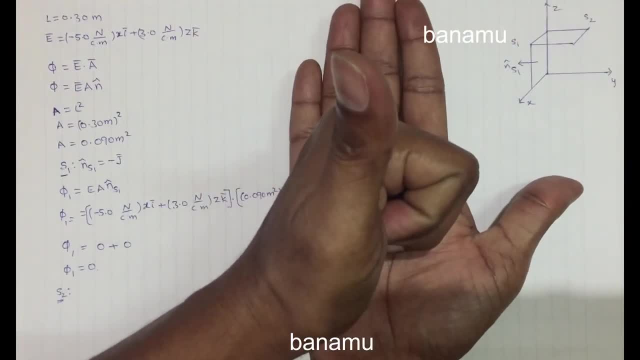 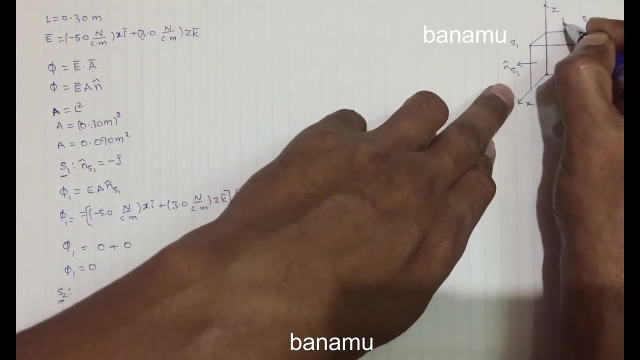 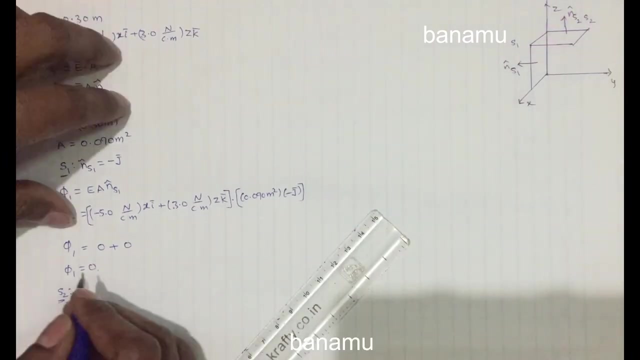 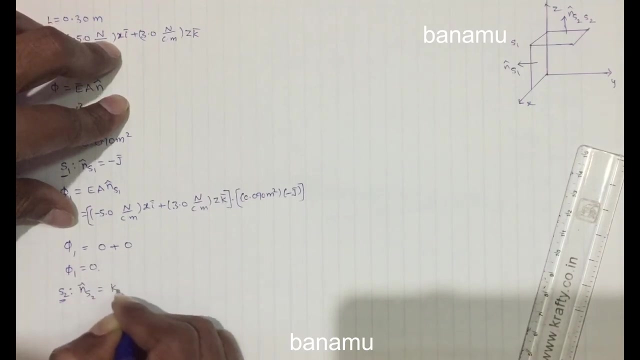 thumb direction is indicated, the unit normal vector of the surface as to. so the direction of the unit normal vector is parallel to the z axis. so this is the n-cap s2, the direction of the unit normal vector along the positive z direction. so the n-cap s2 is taken. the n-cap s2 is equal to k, bar the n-cap s2. 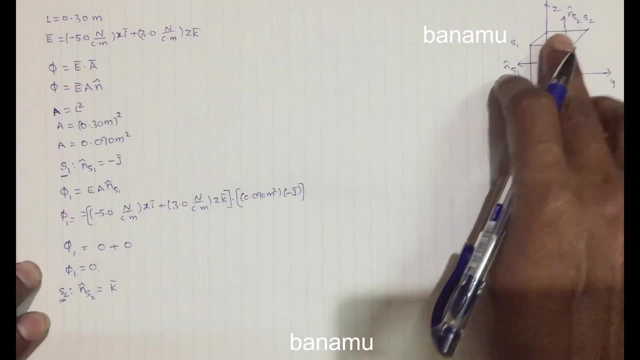 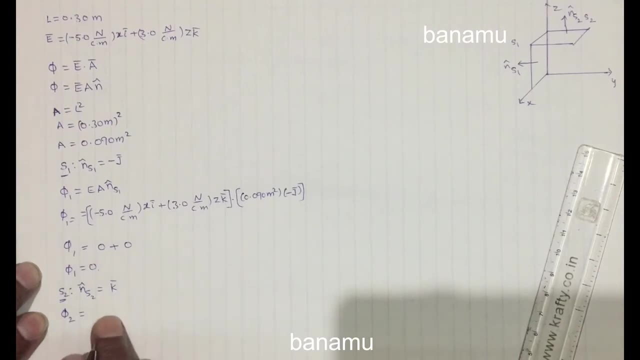 is equal to k bar. so the electric flux at the surface s2 or top of the cube phi 2 is equal to a n-cap s2. so the electric field is the minus 5 Newton per Coulomb meter into X I bar, plus 3 Newton per Coulomb meter into z k bar. this is the electric field. 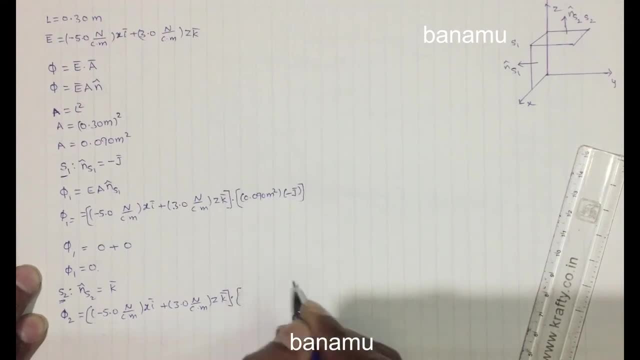 dot. the area of the surface is the zero point, zero nine meter square into the unit. normal vector direction is the along the positive z axis. so k bar. so the electric flux at the surface s2 is equal to phi 2. the dot product of the vectors is i bar, dot k bar is equal to zero. so that is equal to zero plus k bar dot k bar is: 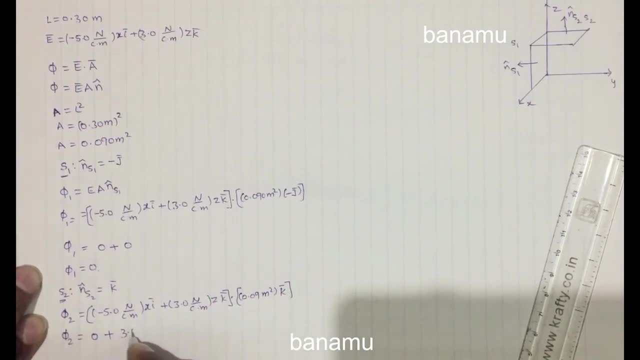 equal to one, so three newton per coulomb meter into z, into 0.09 meter square, so phi 2 is equal to 0.27 newton meter per coulomb, so into z newton meter coulomb into z, so the electric flux at the surface s2 is equal to. 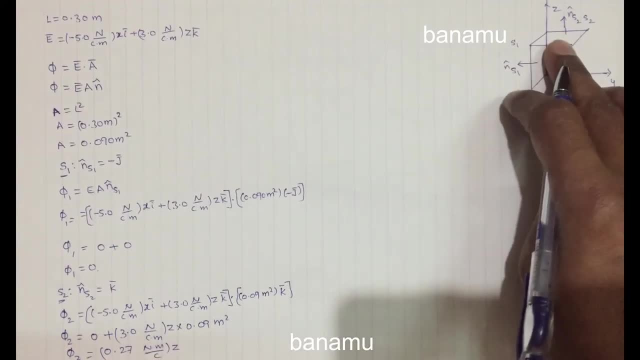 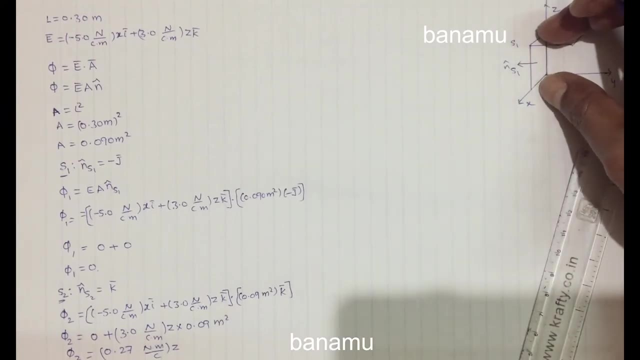 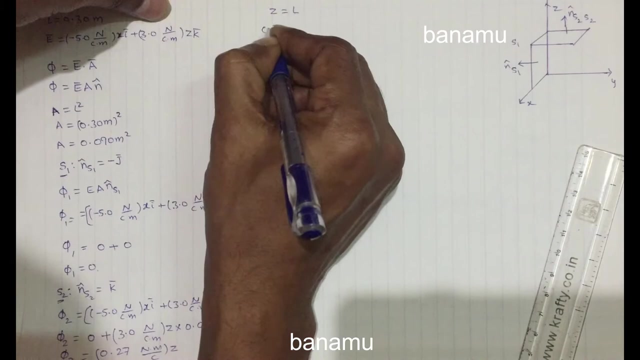 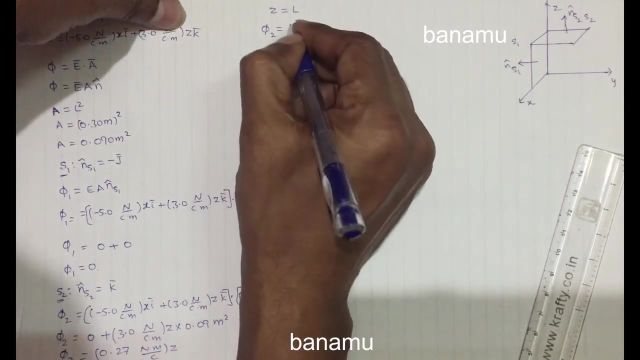 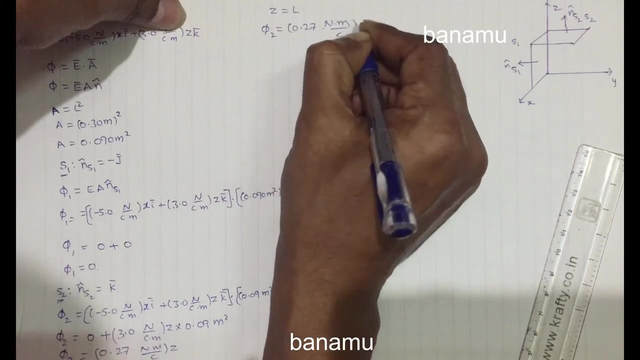 the value of the z is the one side length of the cube, so z is equal to the side length of the cube. this is the z. the length of the cube is l. so where z is equal to l, so the electric flux at the surface S2 is equal to. the value is the 0.27 Newton meter per coulomb into the length Z. 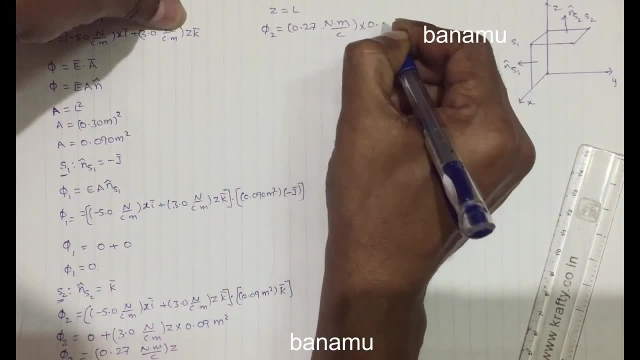 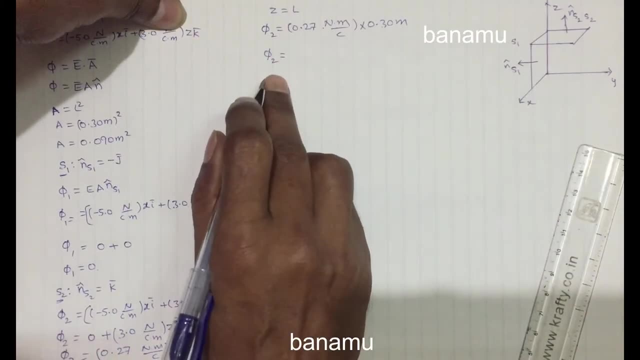 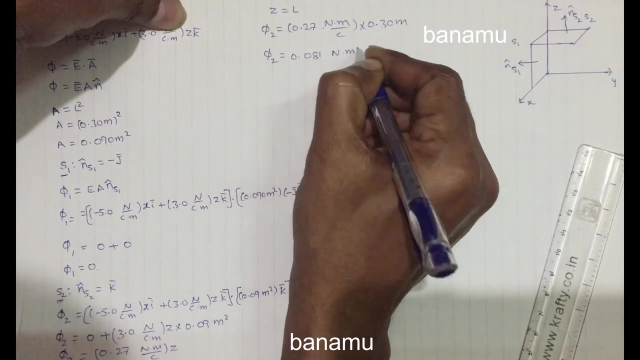 is equal to L, So 0.3 meter. So the electric flux at the surface S2 is phi 2.. Phi 2 is equal to 0.081 Newton meter square per coulomb. This is the flux through the surface S2 or. 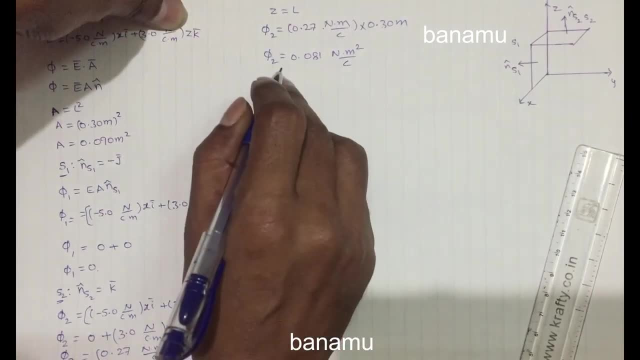 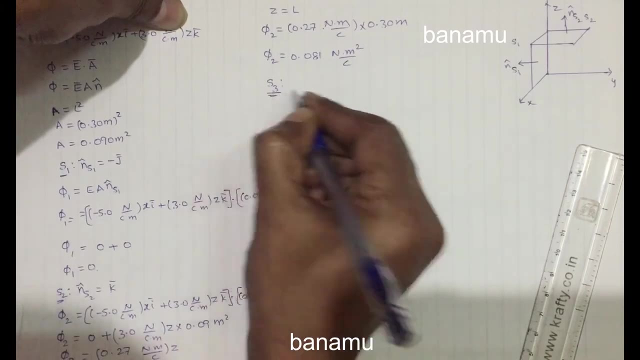 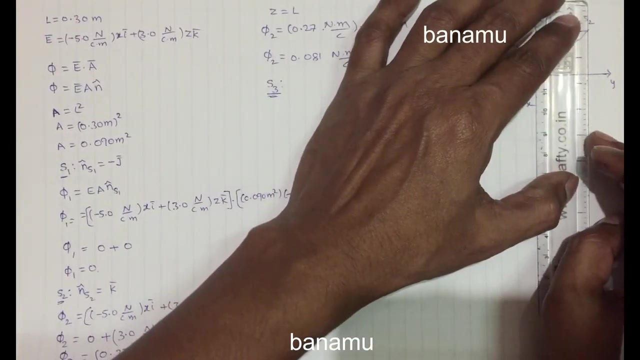 top of the cube And consider the surface S3.. Consider the surface S3.. The surface S3 is the right side of the cube. So this is the right side of the cube. We can draw the surface S2, S3.. 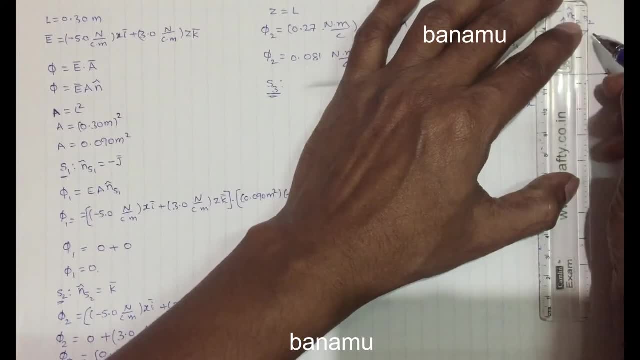 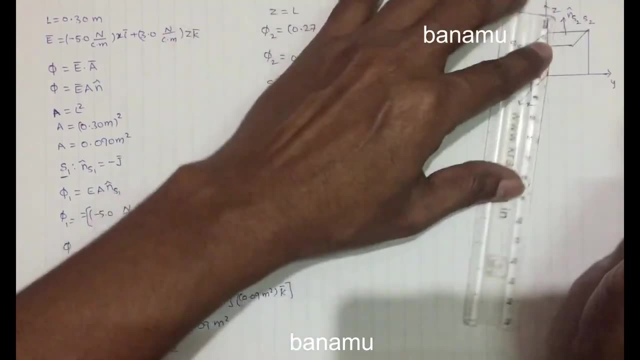 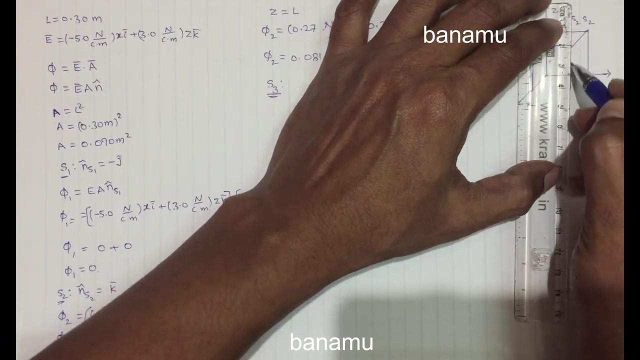 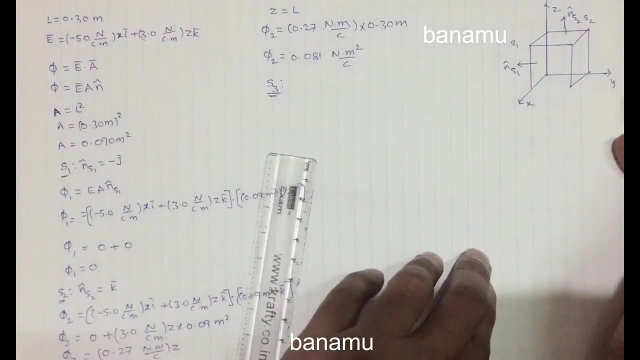 We can draw the surface S3.. This is the surface S3.. We can draw the surface S3.. The surface S3 is the right side of the cube. This is the surface S3.. The surface S3 is the right side of the cube. So this is the surface S3.. 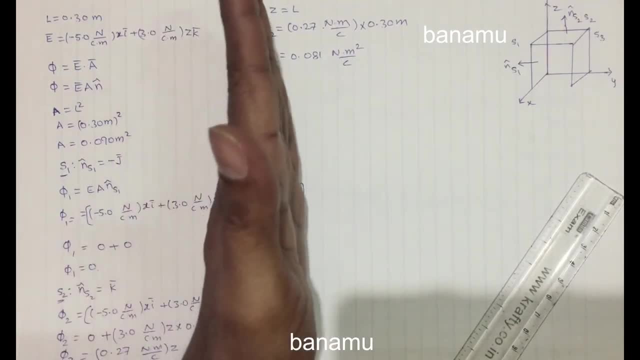 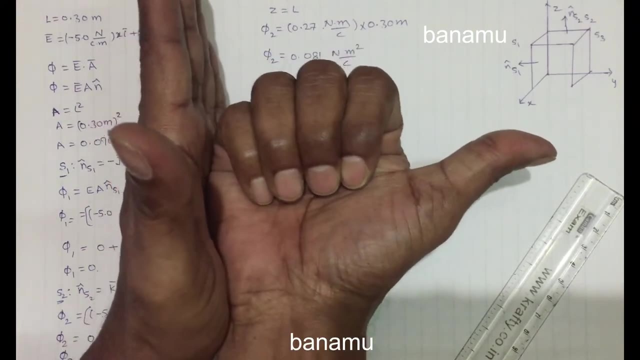 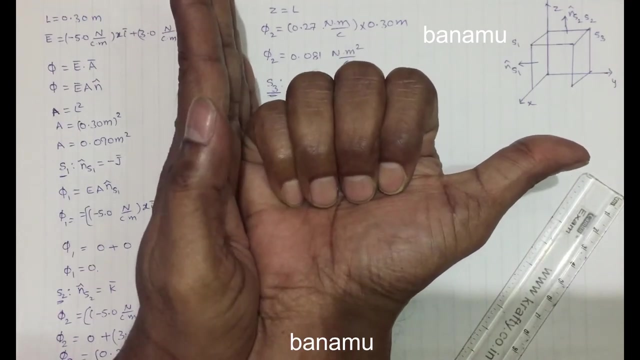 the unit normal vector of the surface S3 is the. this is the surface S3, the unit normal vector of the surface S3 is the direction of the thumb. So this is the perpendicular to the surface. the unit normal vector is perpendicular to the surface S3.. So the direction of the unit normal. 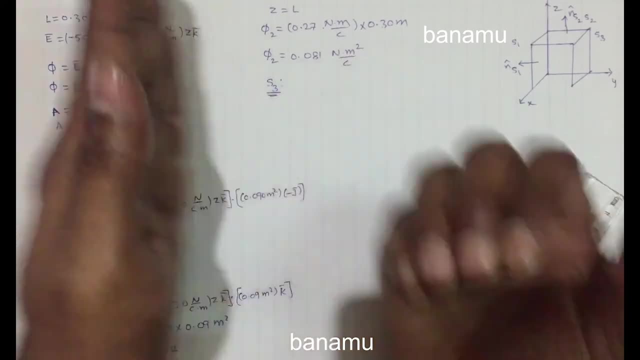 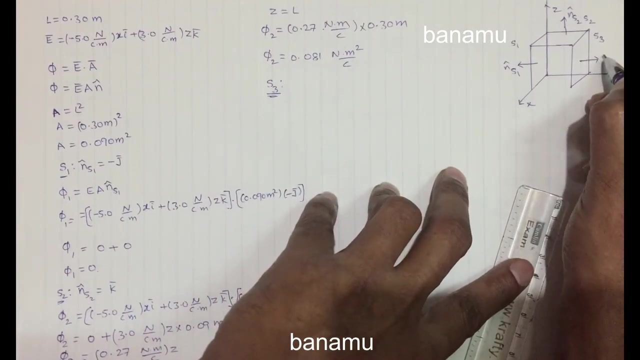 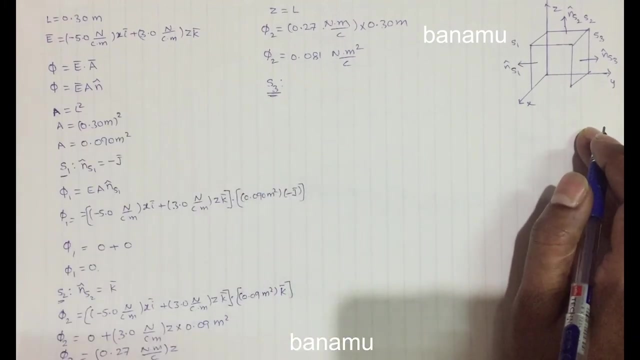 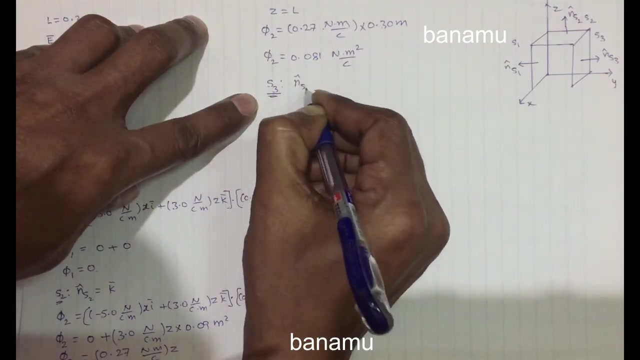 vector along the positive y direction. So this is the. the unit normal vector direction is the this direction: positive y direction. this is the n cap s3, so the direction of the unit normal vector along the positive y direction. so n cap s3 is equal to n cap s3 is equal to plus j bar. 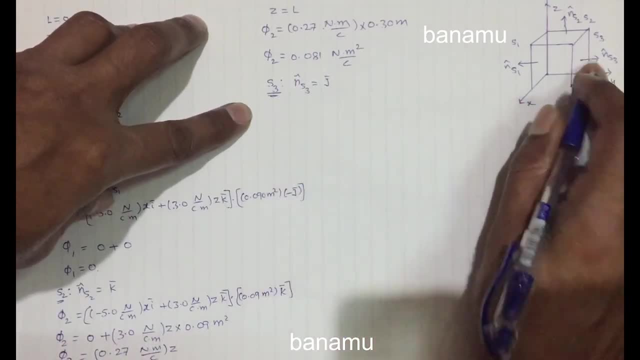 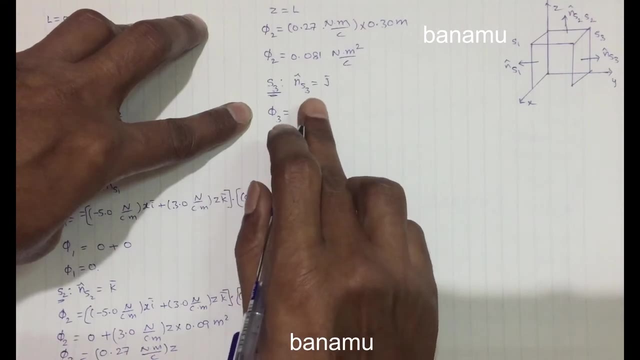 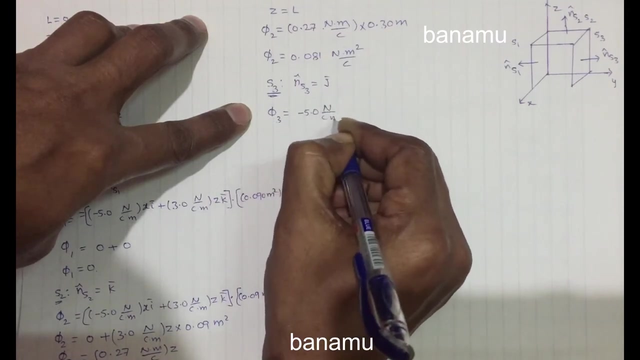 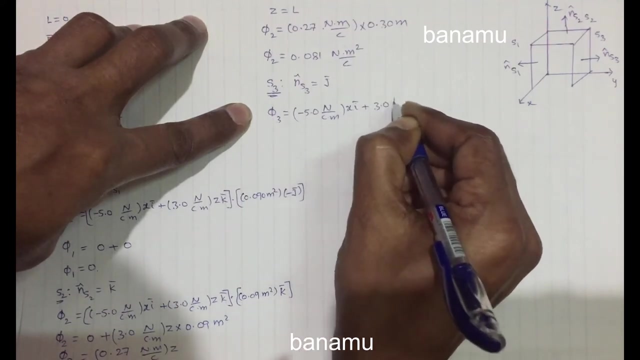 so the electric flux at the surface s3 is the phi 3, phi 3 is equal to e a n cap s3. so the electric field is the minus 5 newton per coulomb meter into x i bar, plus 3 newton per coulomb meter into 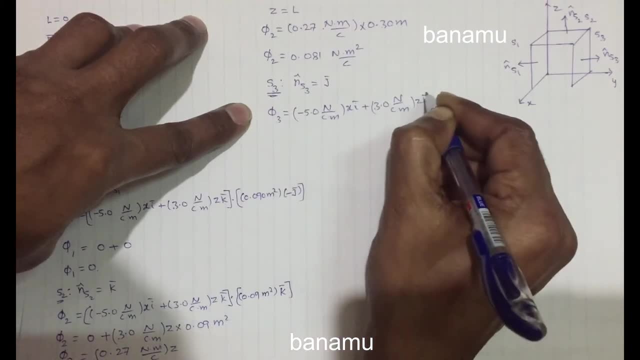 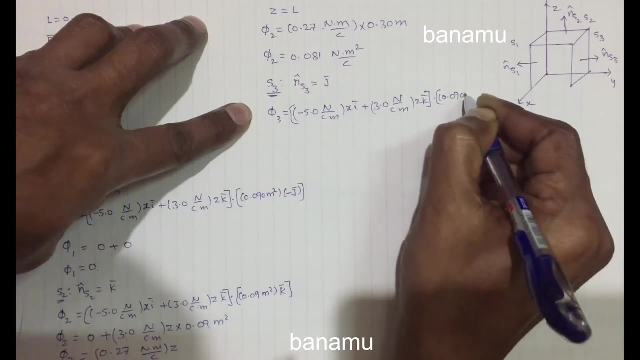 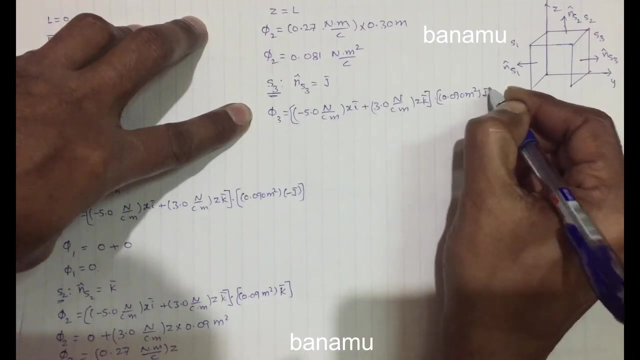 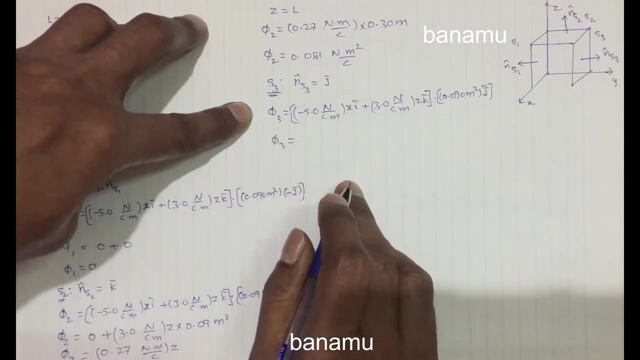 z k bar dot. the area is the 0.09 meter square into the direction of the unit. normal vector is the plus j direction. so phi 3 is equal to the dot product of the two vectors. i bar dot. j bar is equal to 0. 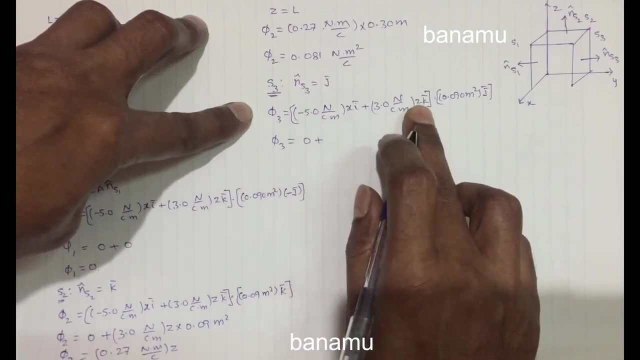 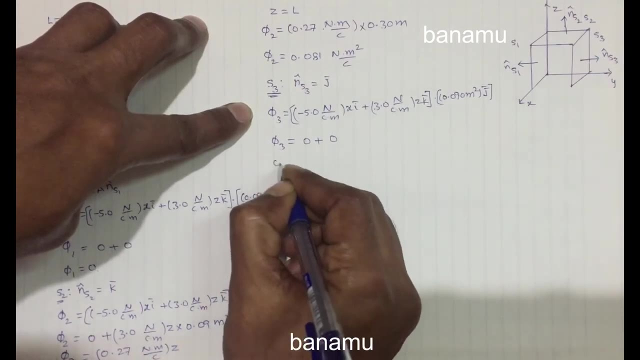 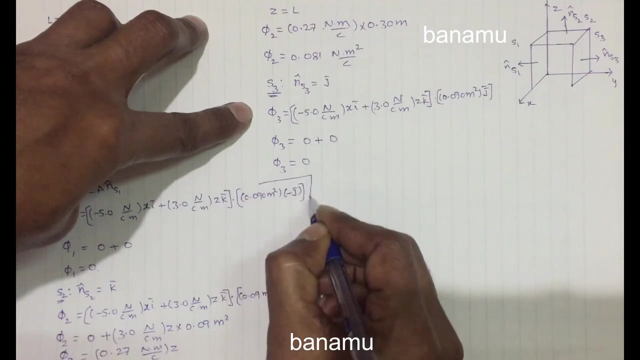 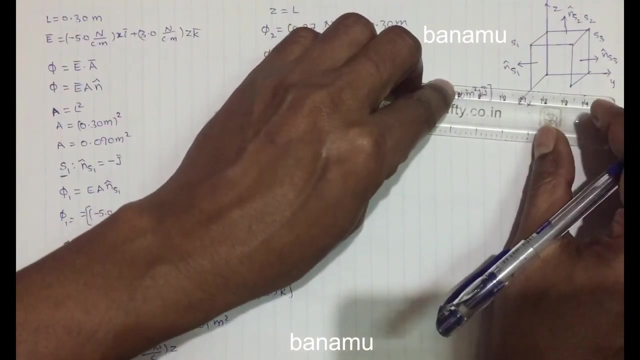 plus k bar, dot j bar is equal to 0. plus k bar, dot j bar is equal to 0. j bar is equal to 0. So the electric flux at the surface S3 is phi. 3 is equal to 0. So we can draw the another surface. Let us surface S4.. The surface S4 is the 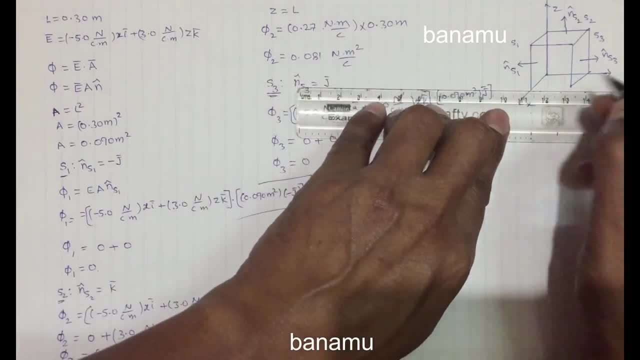 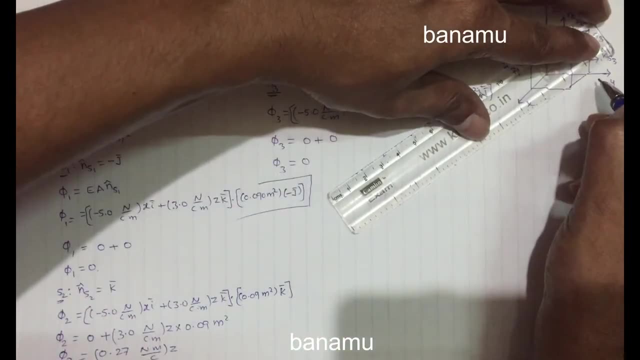 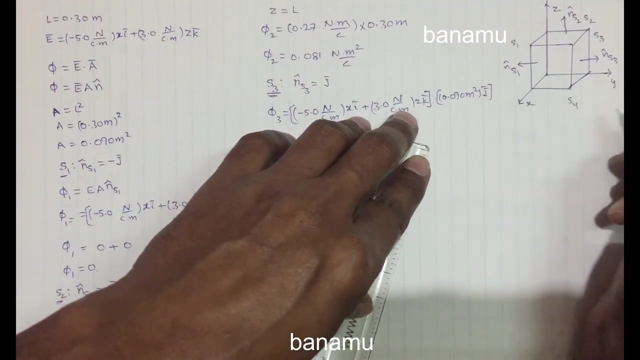 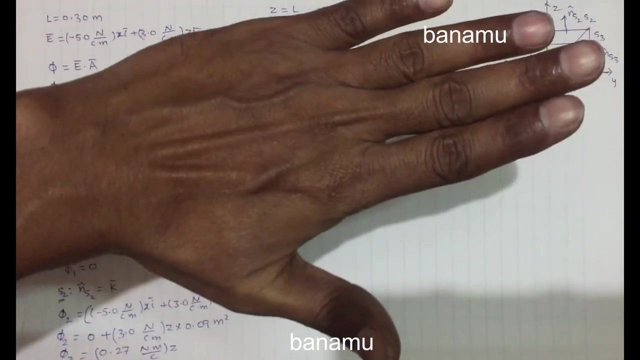 bottom of the bottom of the surface, bottom of the cube, this is the surface S4.. The S4, the unit normal vector of the surface S4 is the. this is the surface S4.. The unit normal vector is the perpendicular to the surface S4.. So the direction from here can now be derived. 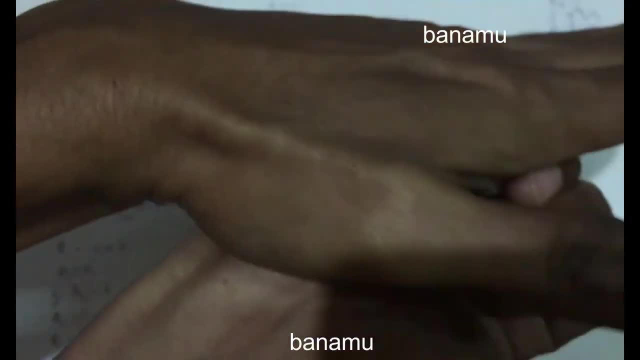 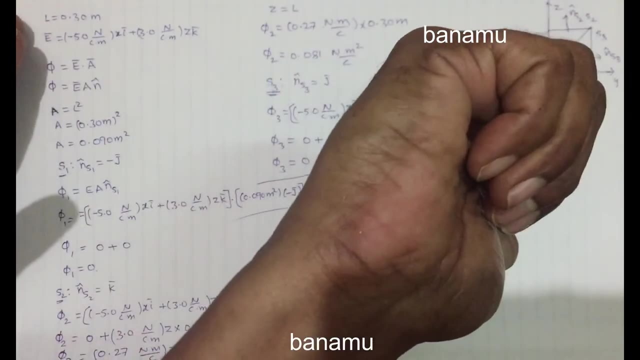 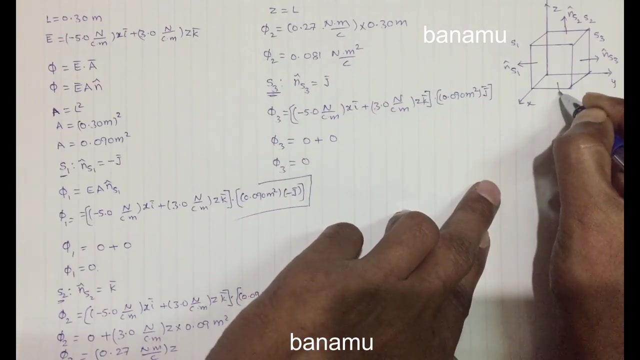 of the thumb is indicated the unit normal vector. this is the direction towards the downwards, towards the downwards. the thumb direction is towards the downwards. this is the the unit normal vector at the surface. S4 is the downwards direction of the cube. this is the n-cap S4, so the unit. 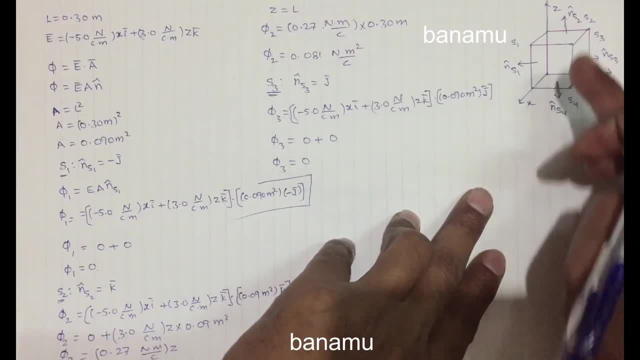 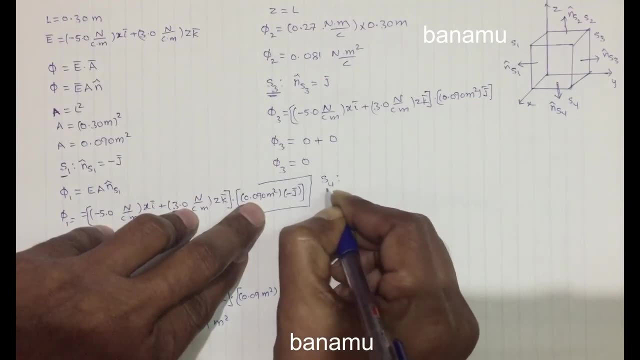 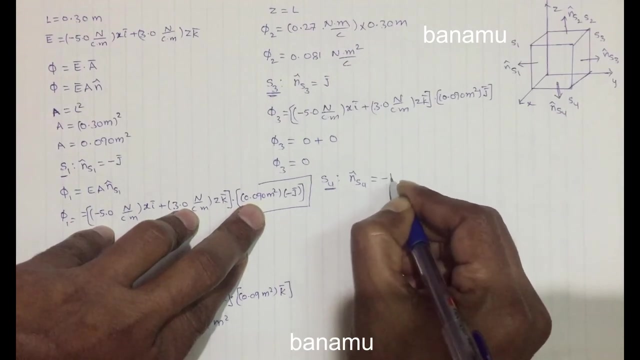 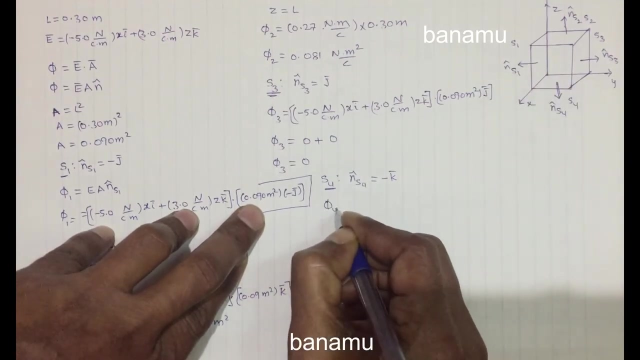 normal vector along the negative z direction. this is the negative z direction. so consider the surface s4, the unit normal vector n cap s4 is equal to minus k bar. the electric flux at that surface s4 is 5, 4. 5 4 is equal to e a n cap s4, so the electric field is minus 5 newton per. 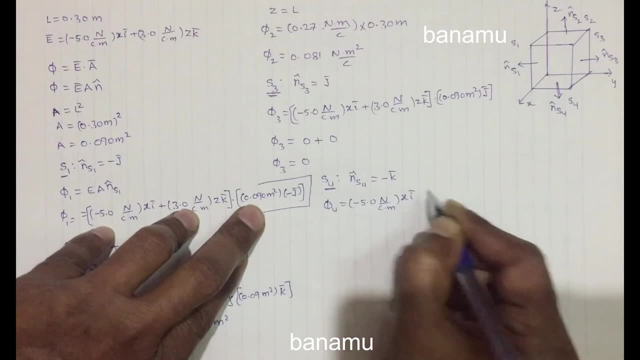 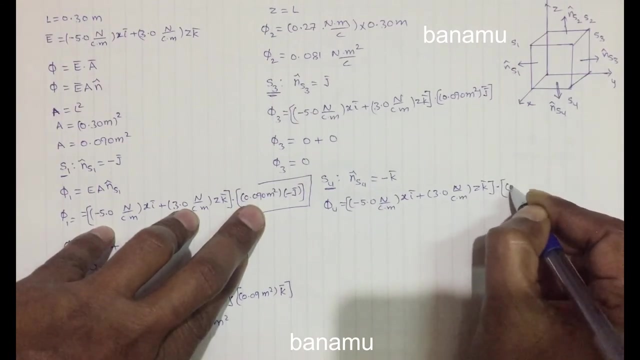 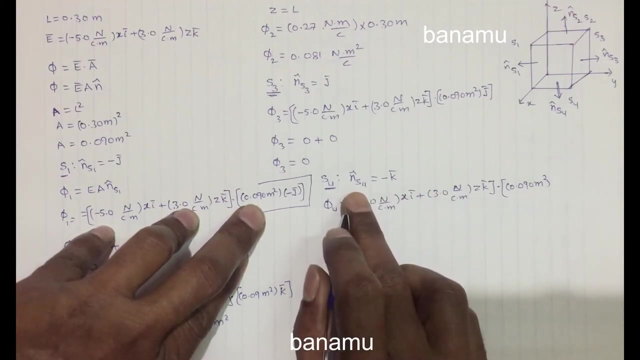 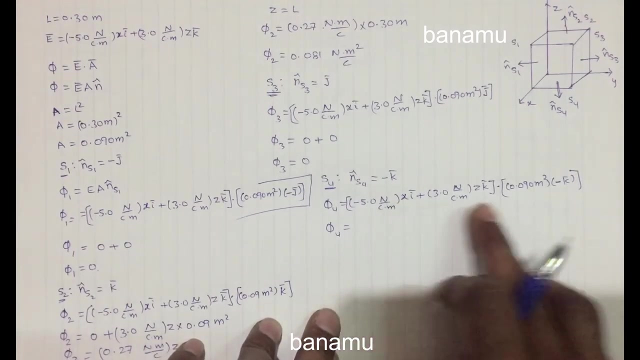 coulomb meter into x i bar, plus 3 newton per coulomb meter into z k bar. this is the electric field dot. the area is the 0.09 meter square into the unit. normal vector at the surface, s4 is the minus k bar, so 5: 4 is equal to the dot. product of the two vectors is the i bar. dot k bar is equal to 0 plus k bar. dot k bar is equal to 1. 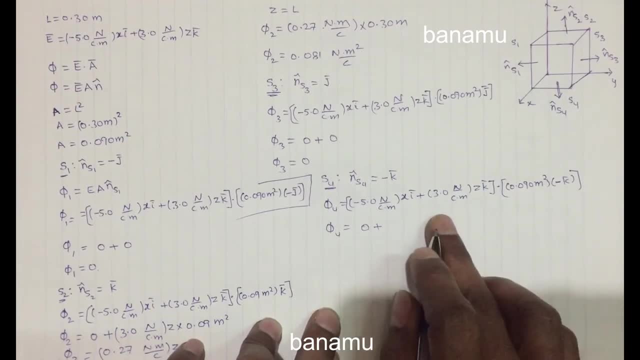 so k bar dot minus k bar is equal to minus one. so that is equal to minus half three into zero point nine. zero is equal to 0.27 Newton meter per coulomb into z, where z is the one cube length of of z, where z is the one cube length of. 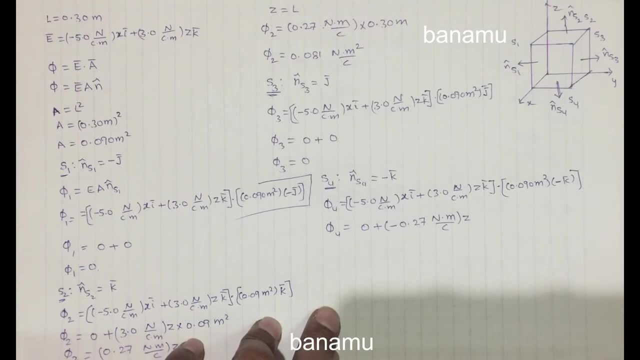 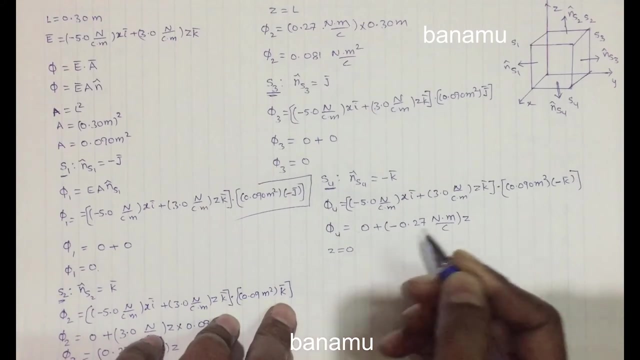 of the one side length of the cube. So in this case the surface S4 are downward of the cube. the length is z is equal to 0 because the cube is placed at the only positive z direction. We have know the negative z, So z is equal to 0 at the bottom of the cube. 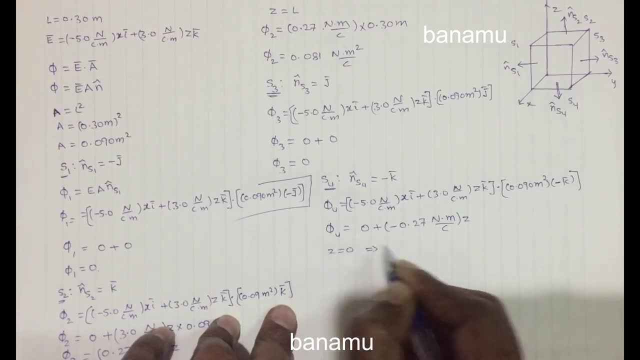 So z is equal to 0.. So in this case the flux 5: 4 is equal to 0 into minus 0.27 Newton meter per coulomb into 0.. 5: 4 is equal to 0.27 Newton meter per coulomb into 0.. 5- 4. 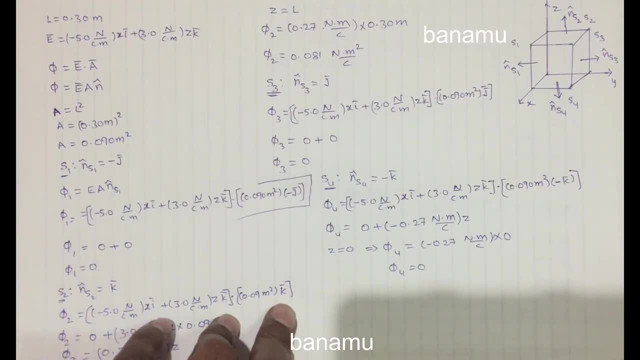 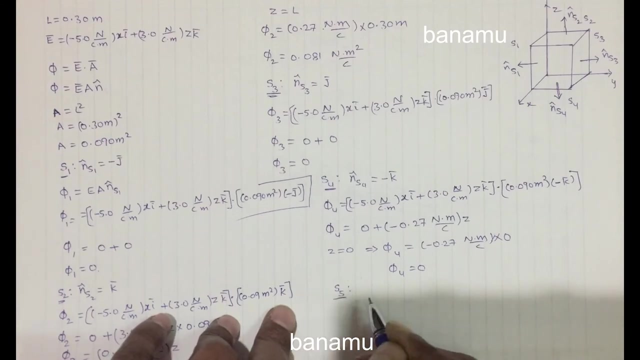 is equal to 0.. So z is equal to 0.. This is the electric flux at the surface, bottom of the surface or surface S4.. We can calculate at the surface S5.. This is the S5.. The S5 is the. this is: 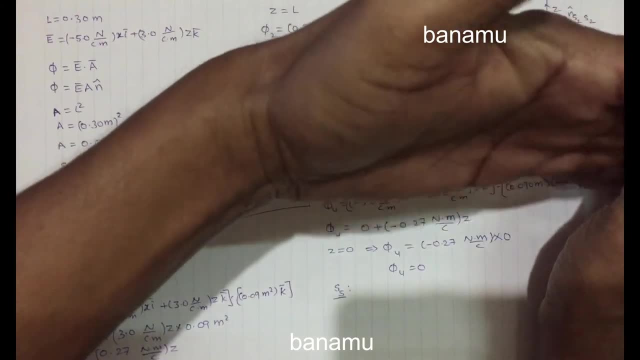 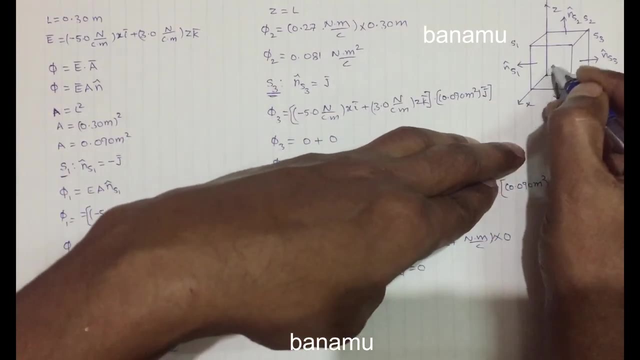 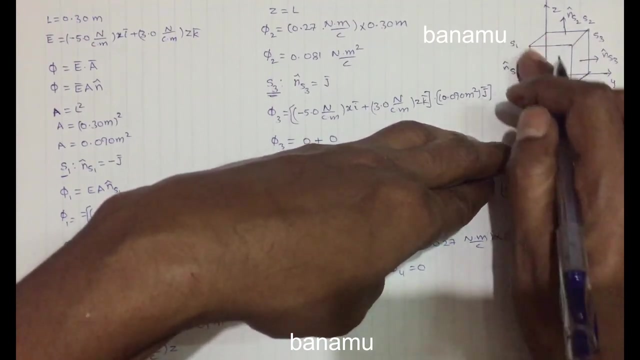 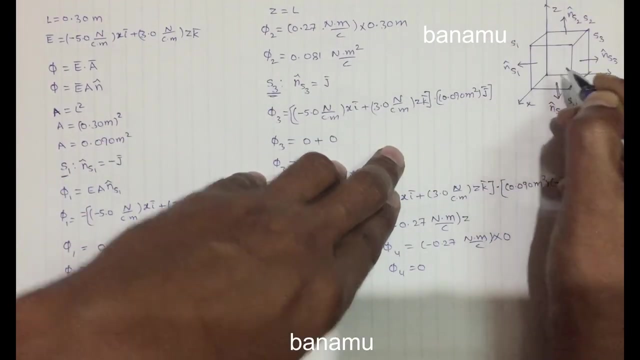 the, the surface. this is the surface S5.. The surface S5, this is the surface S5.. So the direct: this is the surface S5, this is the the surface. this is the Para surface S2, the surface. This is the surface S5. this is the surface S5, the unit normal vectors. 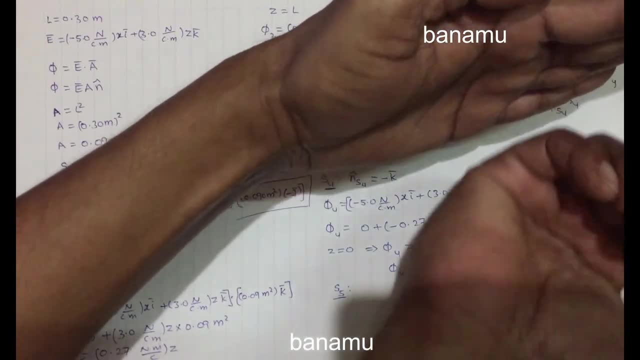 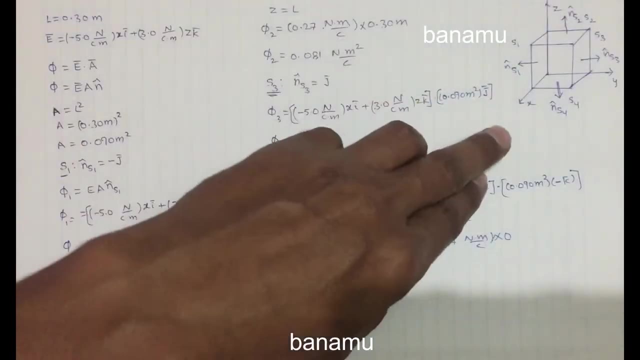 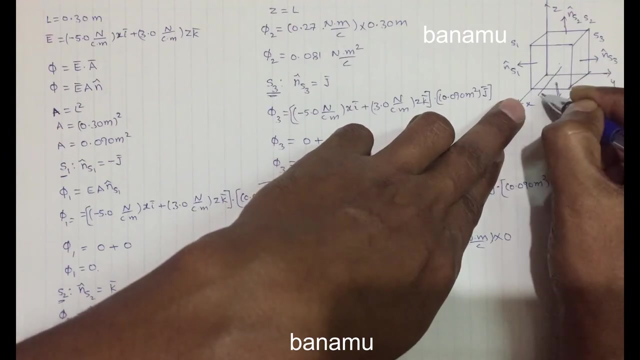 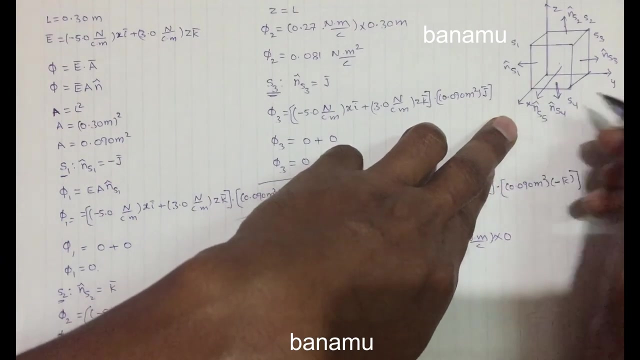 are perpendicular to the surface. So the direction of the unit normal vector is the to the surfaces. So the direction is indicated as the positive x direction. This is the positive x direction. This is the n cap S5.. The surface is indicated as the positive x direction. 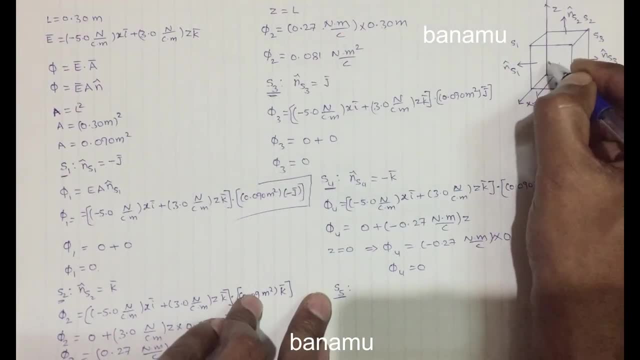 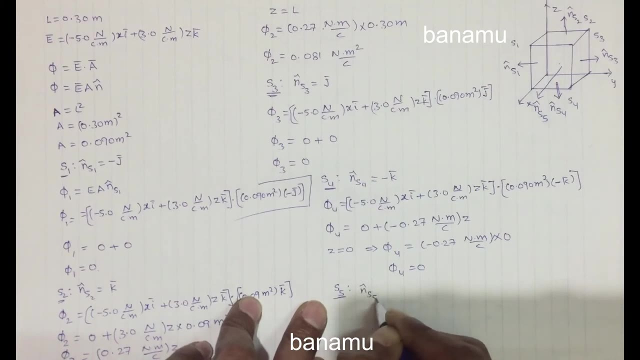 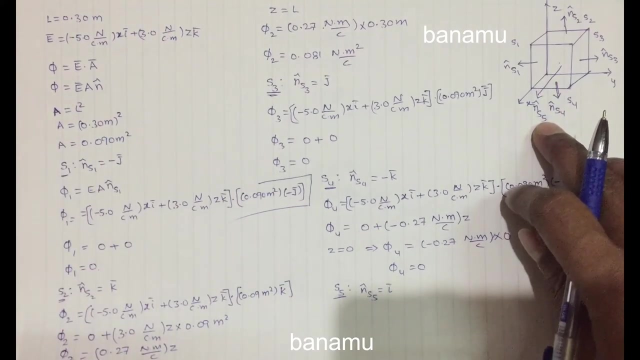 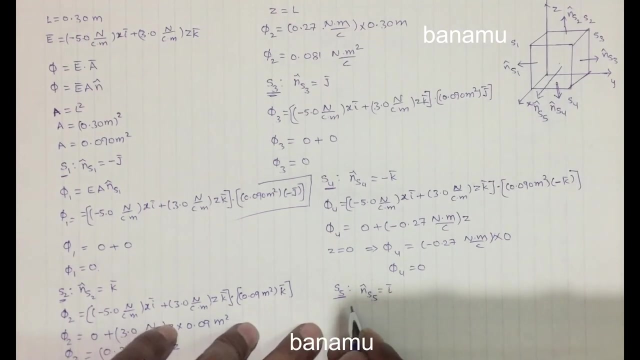 So this is the surface S5.. So the direction indicates the n cap S5 is equal to i bar The surface S5 along the direction of the x axis. So n cap S5 is equal to i bar The electric flux at the surface 5.. 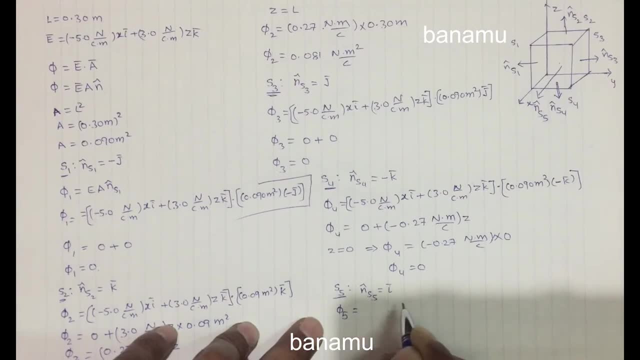 5 is equal to x, is equal to the electric field E, A, n, cap, S5.. So the electric field is the 5 Newton per coulomb meter into x, i bar, plus 3 Newton per coulomb meter into z, k bar dot, the area vector. 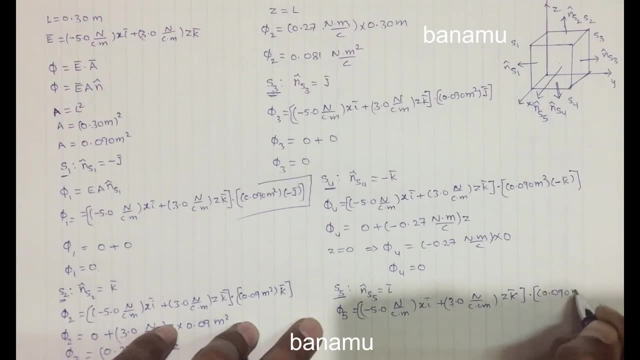 is the 0.09 meter square into the n cap. S5 is the i bar. So 5 is equal to the dot product of the two vectors. So i bar, dot i bar is equal to 1.. So minus 5 Newton per coulomb meter into x. 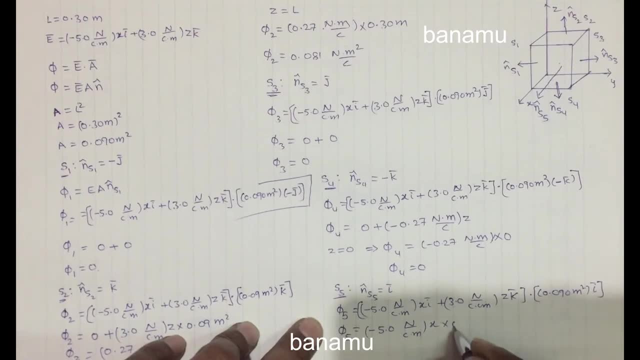 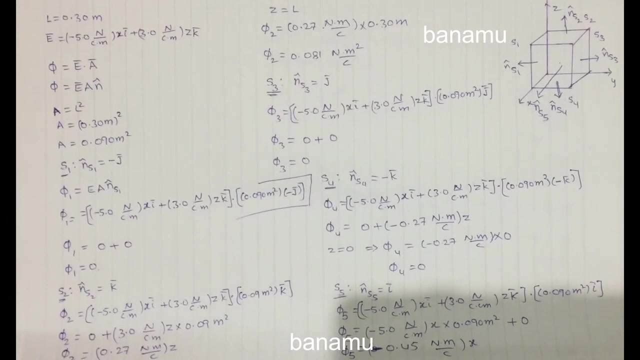 into the area vector is the 0.09 meter square plus k bar. dot i bar is equal to 0. So 5, 5, 5 is equal to 0 point minus minus zero point per 4, 5 Newton meter per coulomb into x, where x is the unit normal vector, where x 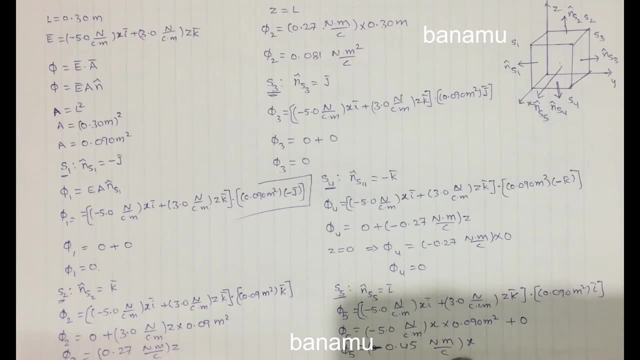 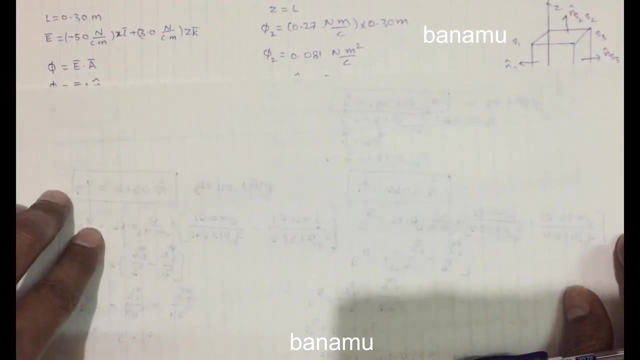 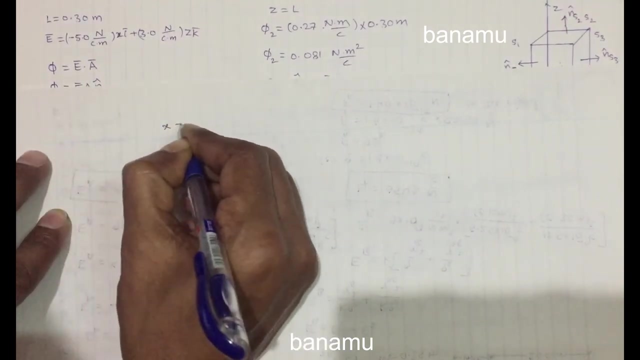 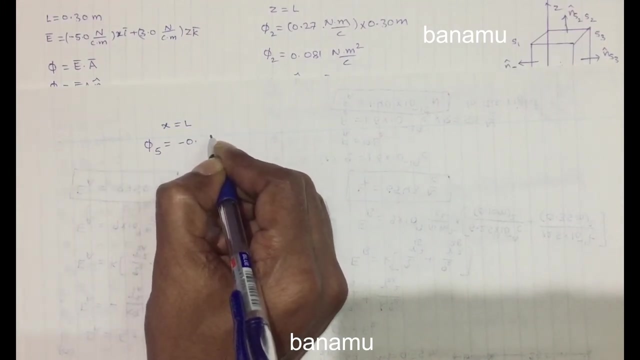 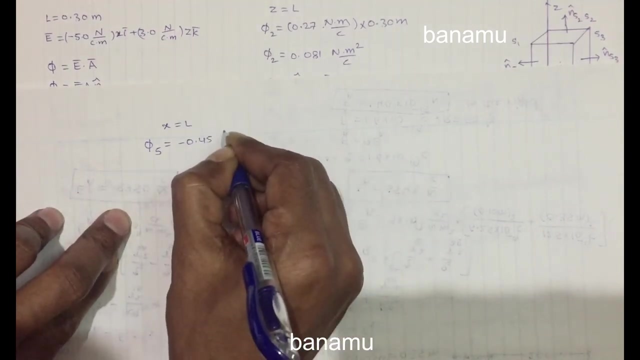 is the one side length of the cube. So the side length of the cube is where x is the one side length of the cube. So in this case, where x is equal to one side length of the cube, x is equal to L. So 5 is equal to minus 0.45 into 0.45 Newton. 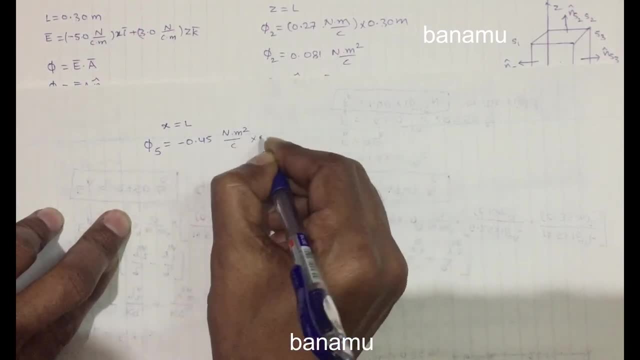 meter per coulomb. So this is the one side length of the cube. So in this case, where x is equal to 1 meter square per coulomb into the side length is the 0.3 meters, So 5, 5. 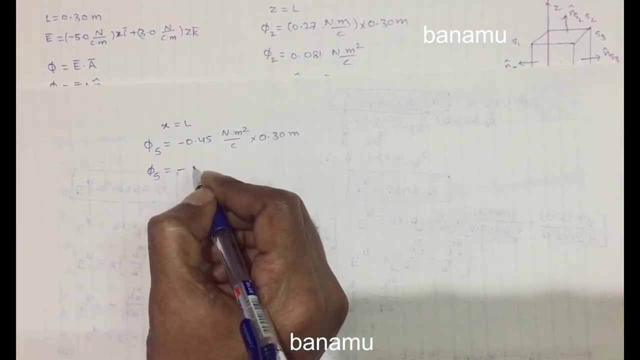 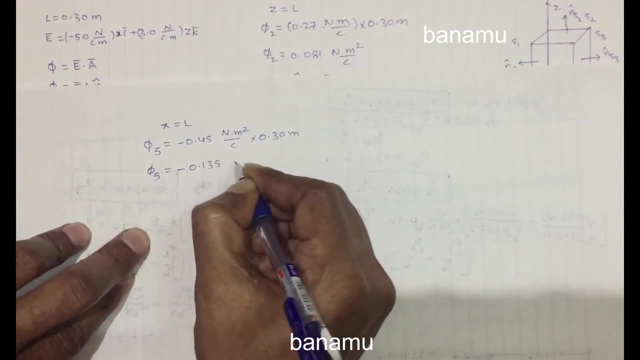 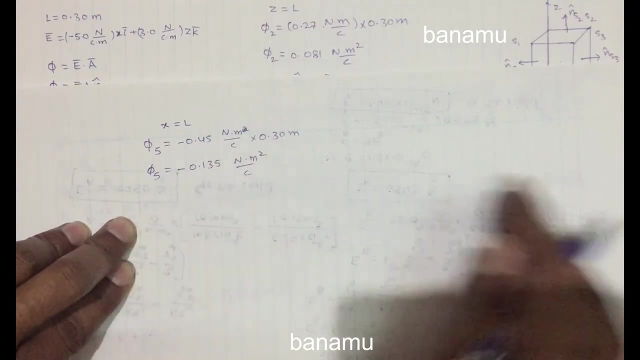 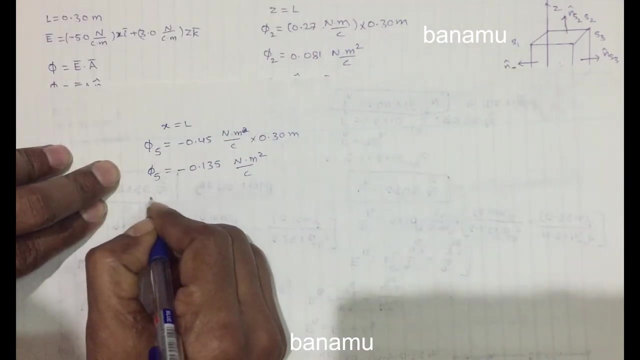 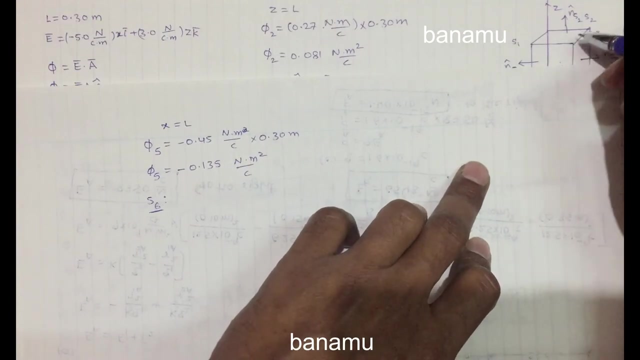 is equal to minus 5,. 5 is equal to minus 0.135 Newton meter square per coulomb. Newton meter square per coulomb. This is the electric flux at the surface 5.. And consider the surface S6.. This is the outside of the cube. This is the outside of the cube. This cube is indicated. 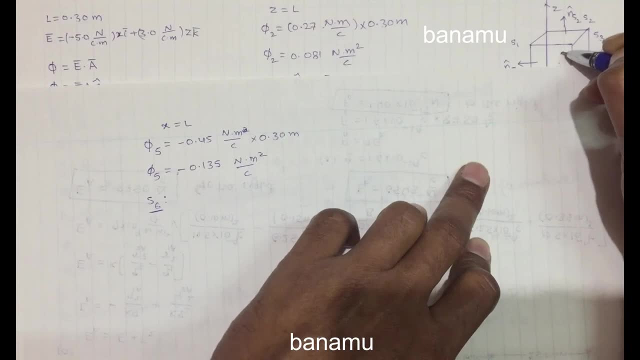 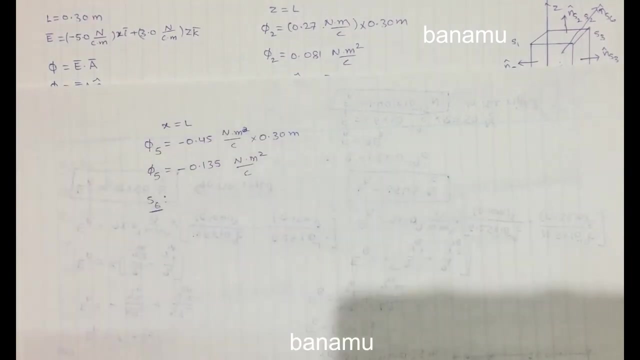 as the surface. So the direction is: this is the. this direction. This is the n cap S6.. This is the n cap S6.. This is the n cap S6.. So the direction of the n cap S6.. This is the, this is the surface 6.. So the direction. 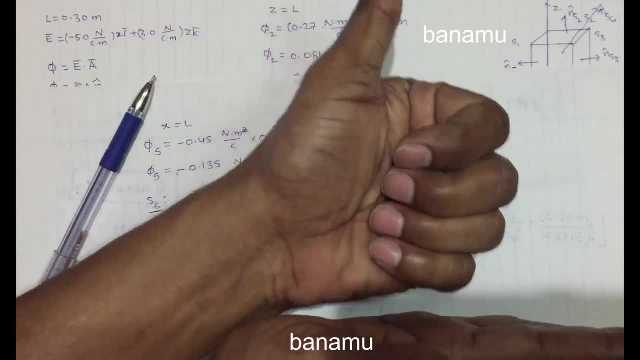 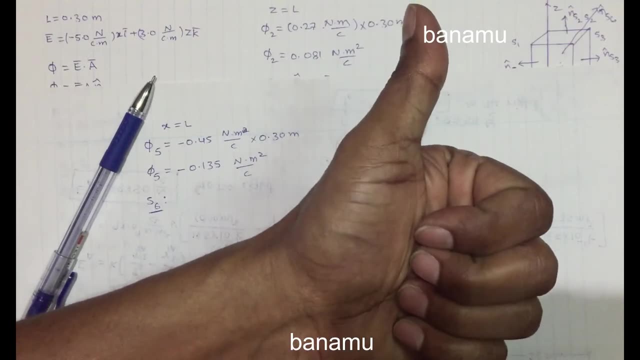 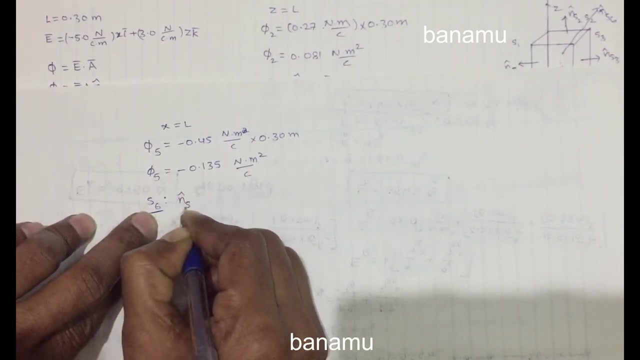 of the now unit normal vector is perpendicular to the surface. So the direction is taken, the negative x direction. So the surface n cap, the surface n cap S6 is equal to: this is the'll height minus 1 meter square. This is the n cap, this square, This is the number. 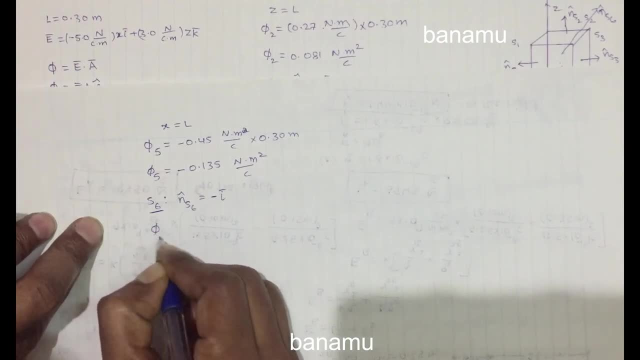 s is equal to minus i bar. So the electric flux at that surface 5, 6 is equal to the electric field e A n cap S6.. So the electric field is the minus 5 Newton per coulomb m. 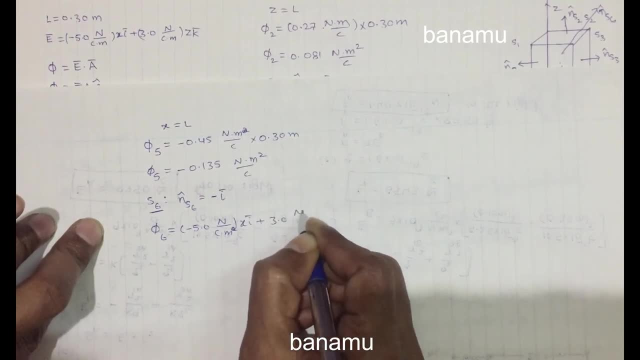 meter, okay, into x i bar Number s is equal to Minus n cap. Therefore the electric b overcome the electric flux at that surface. 5.6 is equal to E A n cap, S6.. So the electric field is the minus 5 Newton per coulomb meter into x i bar, plus 3 Newton per. 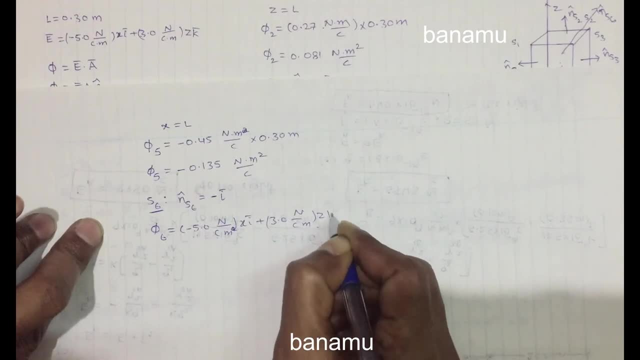 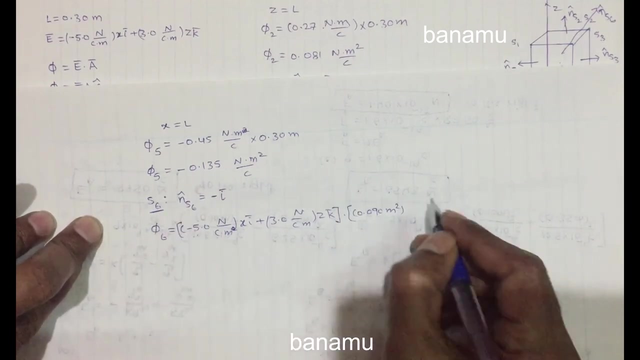 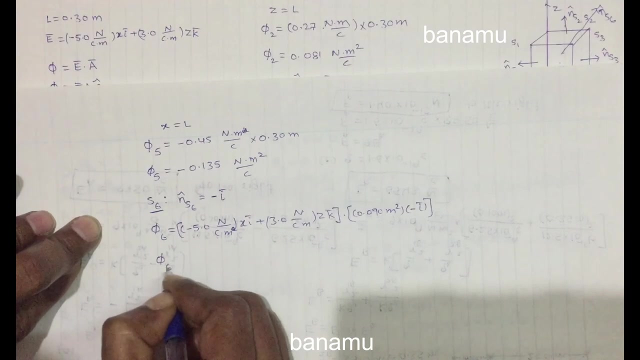 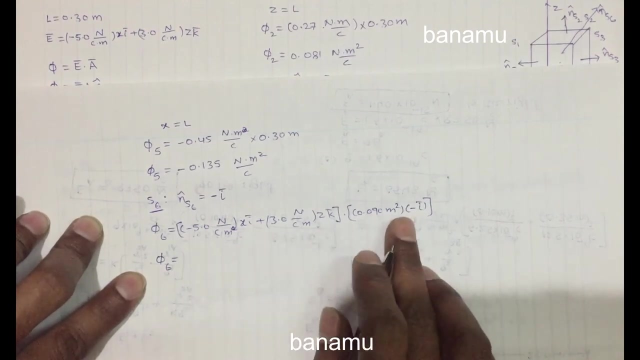 per coulomb meter into z k bar dot. the unit area vector is the 0.09 meter square into the unit normal vector n cap S6 is the minus i bar. So in this case the electric flux at the surface S6 is the 5- 6. the dot product of the vector is the i bar dot. i bar is equal to 1.. 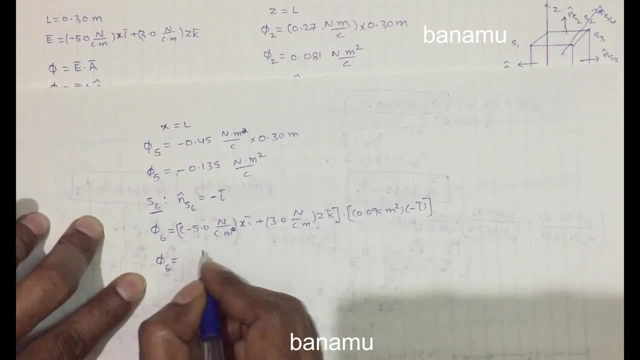 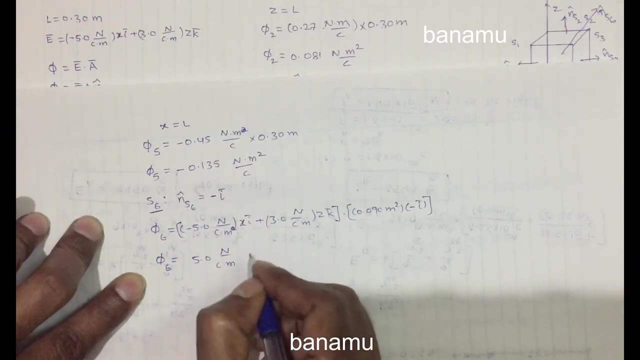 So minus into minus plus, in this case 5 newton per coulomb meter into x into 0.09 meter square. So 5: 6 is equal to 0.45 newton meter per coulomb into x. So in this case the 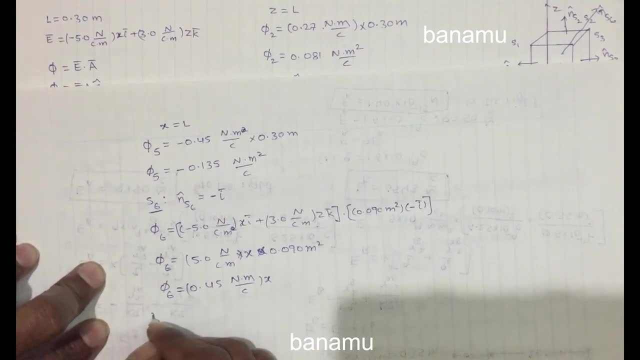 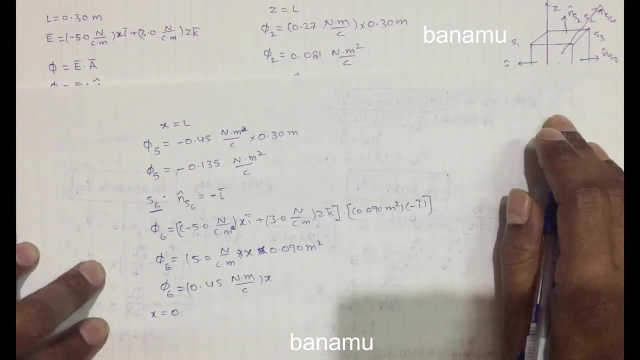 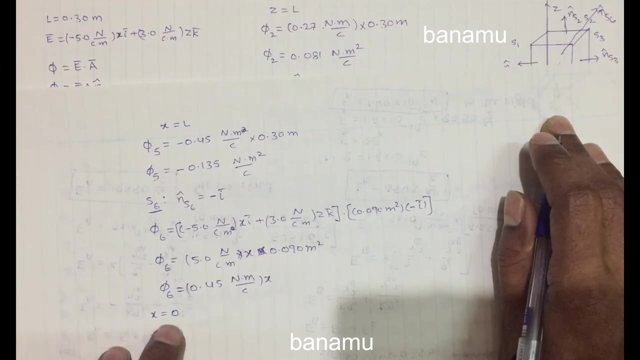 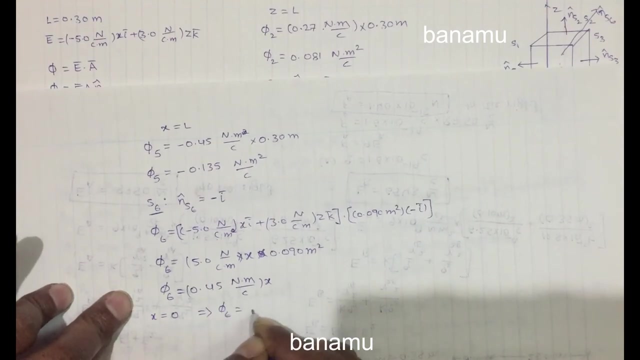 length of the x. the length of the x. x is equal to 0 because 0 because the cube is placed at the only positive x axis only. So in this negative x axis, x is equal to 0. So the electric flux, at this case 5, 6, is equal to 0.45 newton meter per coulomb into 0. The flux. 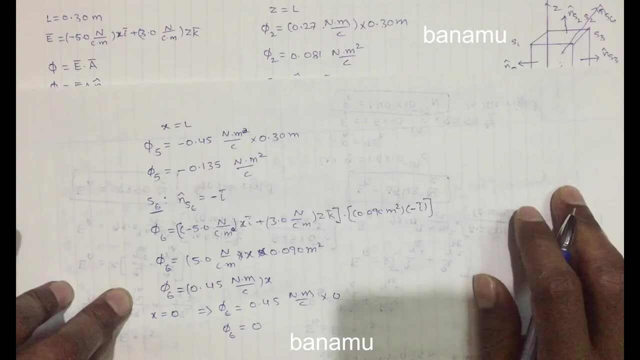 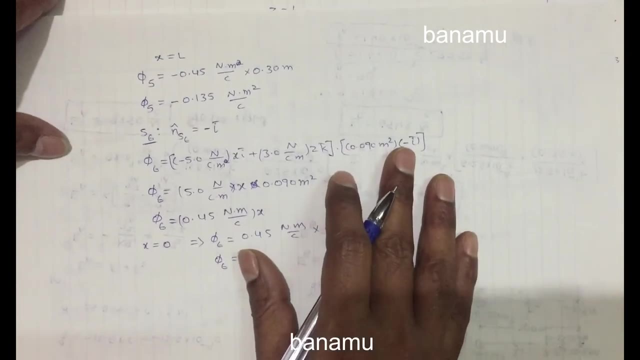 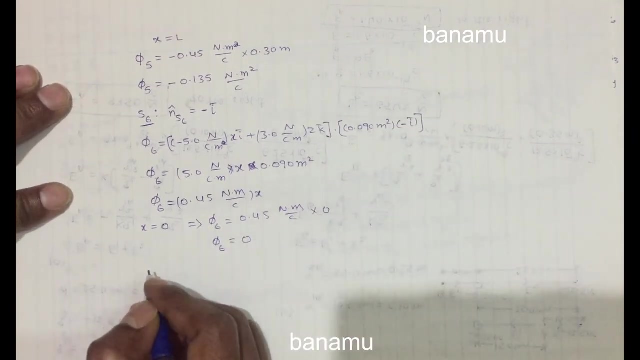 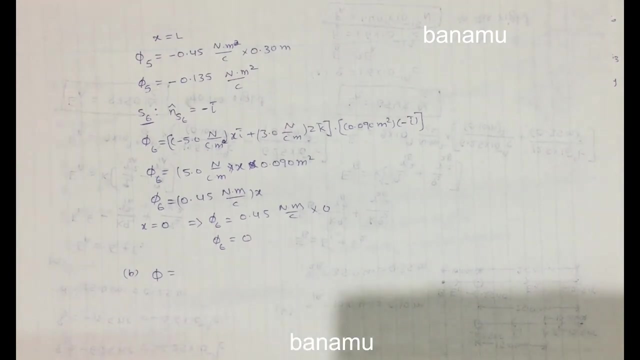 5, 6 is equal to 0 at the surface S6. this is the flux at the surface x 6.. We can calculate the part b. we can calculate the part b. the electric, the total flux in the cube is phi is equal to. we can calculate the. 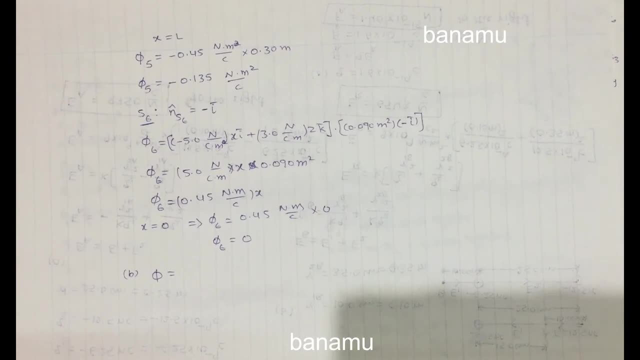 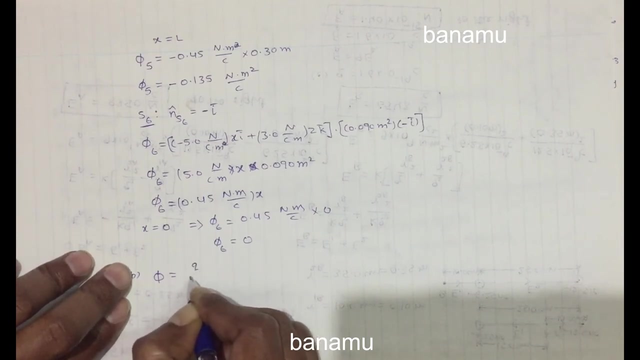 part B. The part B is the total electric charge inside the cube. So according to the Gauss law, the flux phi is equal to the charge inclined surface Q by epsilon. naught From this equation, the charge inclined the surface Q is equal to the charge inclined the surface Q is equal. 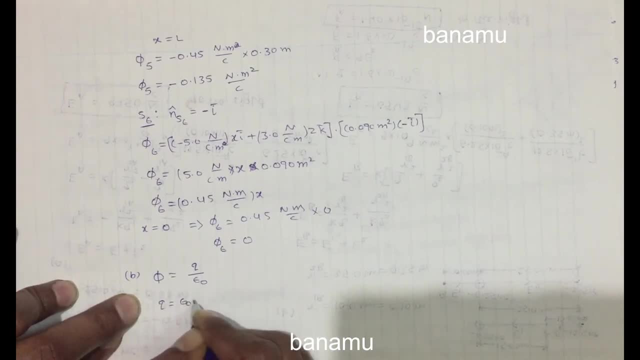 to epsilon naught phi. So where phi is the total flux of the surface, the total flux phi is equal to phi 1 plus phi 2 plus phi 3 plus phi 4 plus phi 5 plus phi 6.. This is 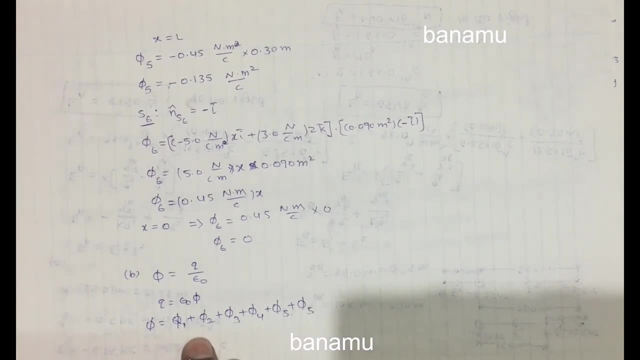 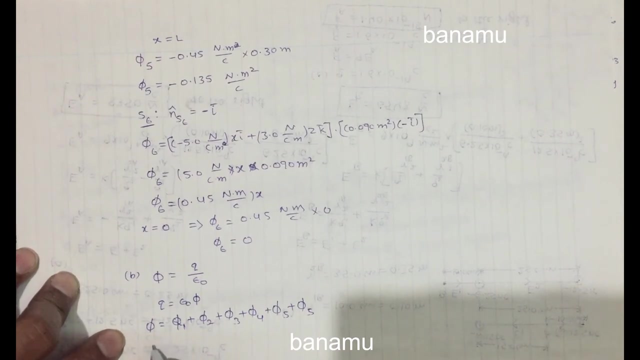 the sum of the charge Each, the flux through the each phase, the sum of the flux through the each phase. So in this case the total flux phi is equalled. in this case the total flux phi is equivalent. phi 1 is 0 plus phi 2.. Phi 2 is the 0.081 Newton meter square per coulomb minus Qn. 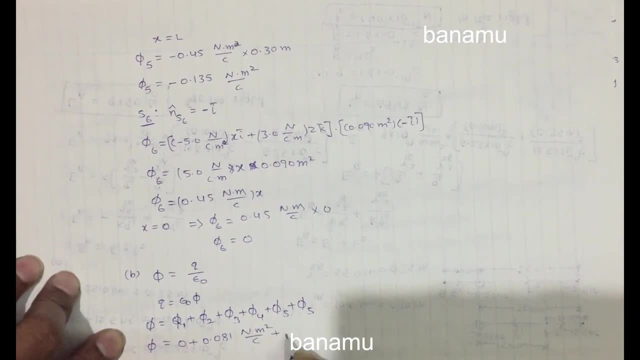 plus 53,. 53 is the 0,. plus 54, 54 is the 0,. 55, 55 is the minus 0.135 Newton meter square per coulomb, plus 56 is the 0.. The total flux in the surface is the 5 is equal to the total flux. 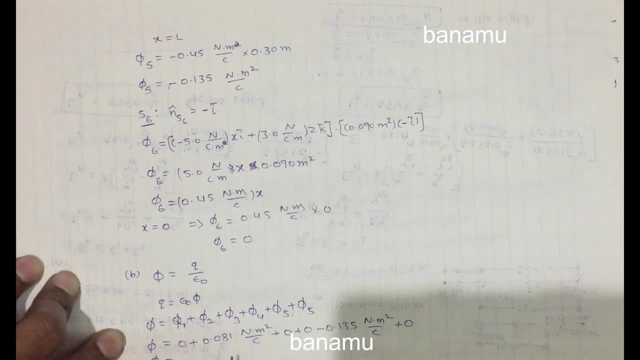 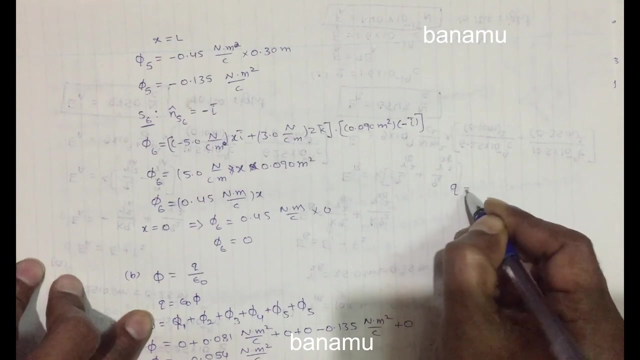 in the surface. 5 is equal to minus 0.054 Newton meter square per coulomb. This is the flux through the surface. We can calculate the charge inclined inside the cube. Q is equal to. Q is equal to epsilon naught 5.. So the value of the epsilon is the 8.854 into 10 to the power of minus 12 coulomb. 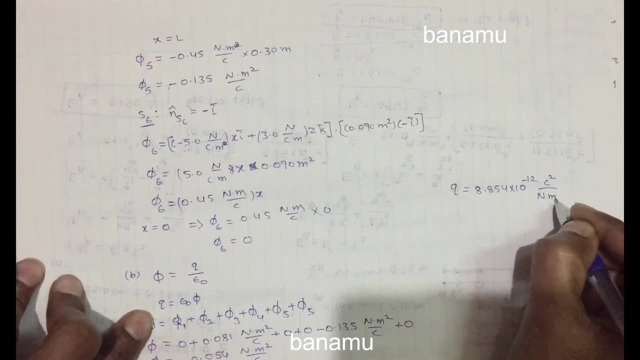 square by Newton meter square into The total flux is the minus of 0.054 Newton meter square per coulomb. So the charge inclined in the surface is equal to minus 4.78 into 10, to the power of minus 13 coulomb. 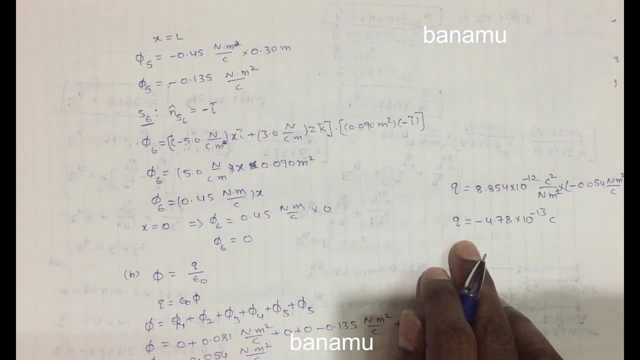 So this is the charge inside the cube of the, the charge in the inclined charge inside the cube. So the negative indicates the, the electric field, the flux through the inside the cube is taken the negative and the flux through the out of the surface is taken the positive.